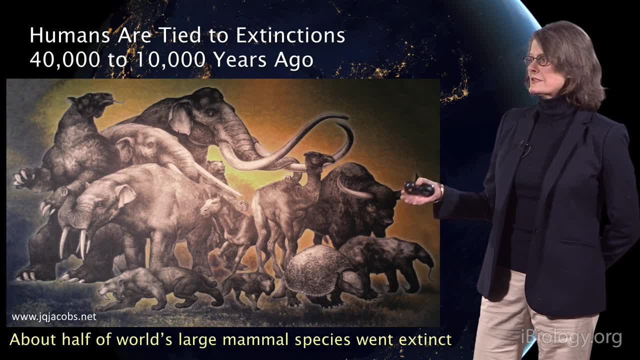 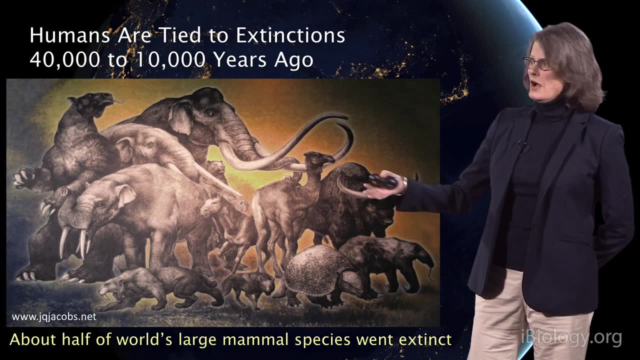 So this expansion was also tied to to extinctions of large animals, So we call this the Late Pleistocene megafaunal extinction. And in addition to the loss of these animals, for example, all of which were present in North America until about 10,000 years ago, 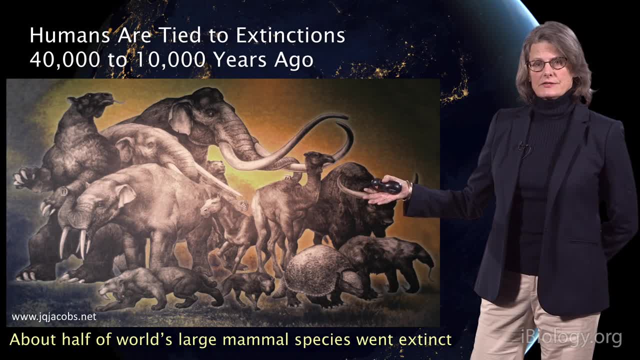 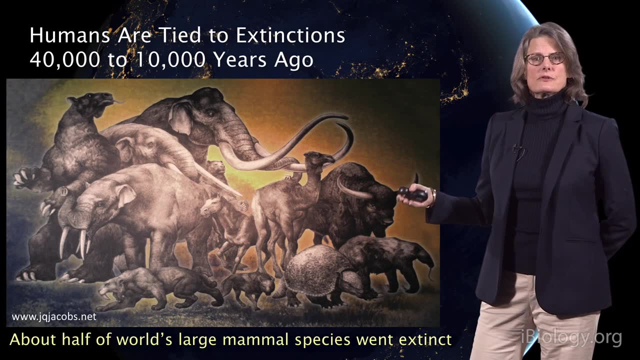 10,000 years ago there was also a climate warming event. So not only the expansion of humans, but also this climate change that happened at the same time. It turns out those are exactly the same two features that are affecting the planet today. 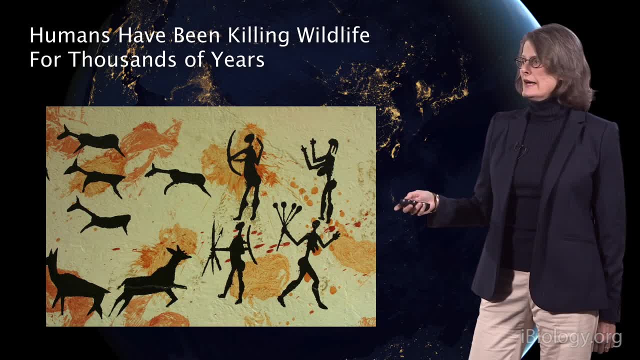 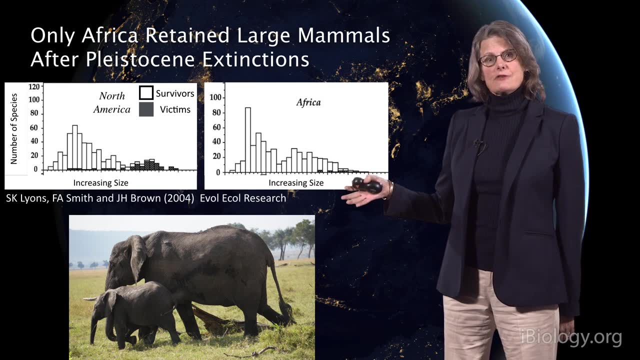 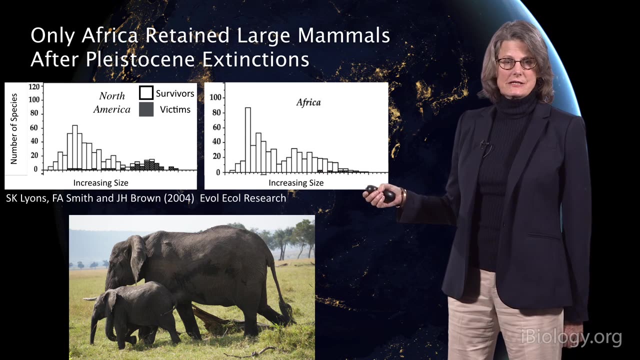 Humans, in fact, have been killing, deliberately killing wildlife for thousands of years And through that, that expansion out of Africa, it turns out that every continent lost their large animals, Not just North America. What you see here are bar graphs of just the number of species in different size categories. 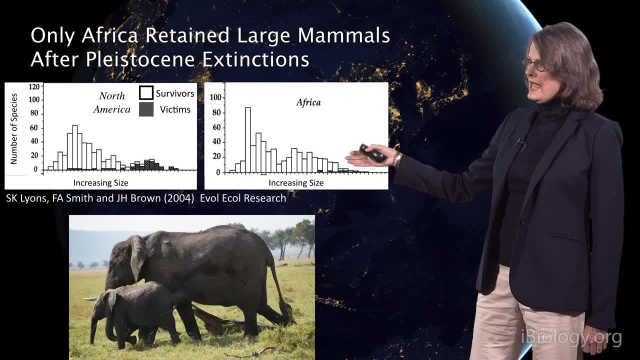 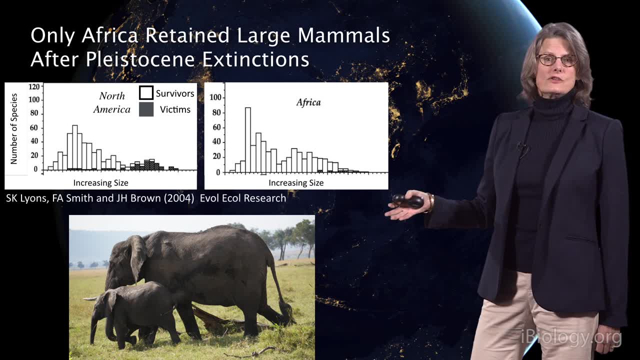 So over here are the smaller animals and over here are the larger animals. In Africa, it's really the only continent that maintained most of the large animals, like we see these elephants today, whereas in North America and the other continents lost their megafauna, lost their large animals. 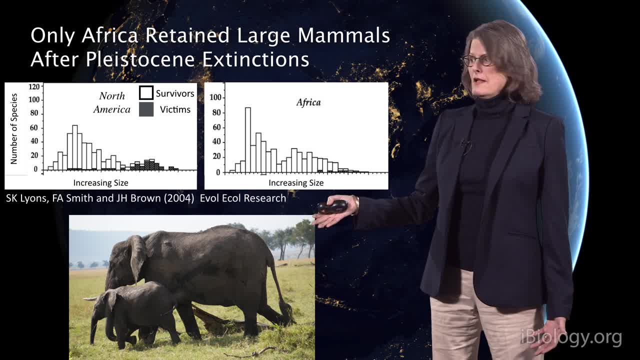 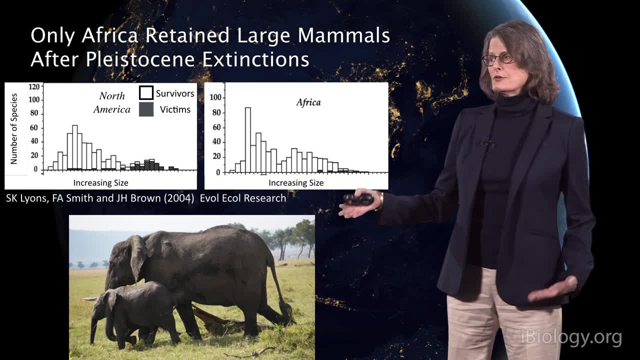 These elephants, though, now are threatened with extinction as well. They have a gestation time of 22 months and, on on average, one elephant has killed every 15 minutes. There's no way that this large, slow metabolism animal could actually keep keep up with. 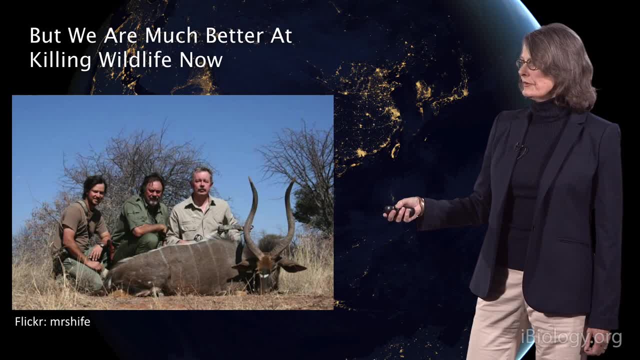 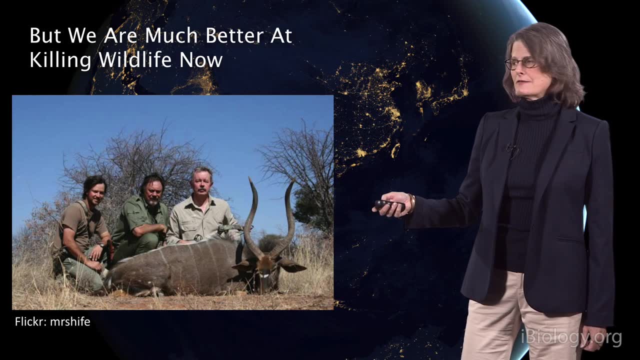 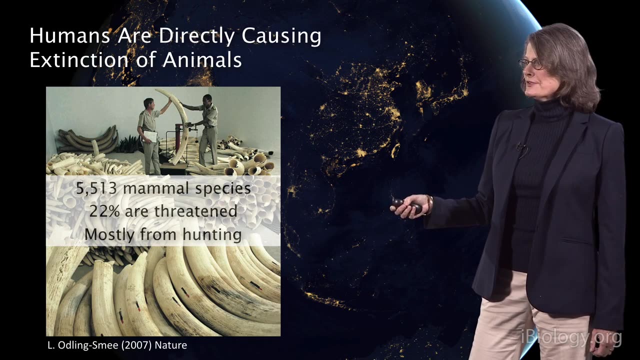 the deliberate slaughter of these animals. We're much, much better at killing wildlife. As a matter of fact, we specialize in going after the very last of some of these exquisite animals. So, among about 5,500 mammal species, almost a quarter of them are threatened, and most 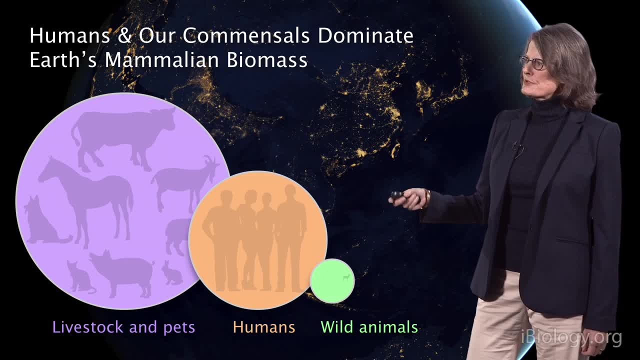 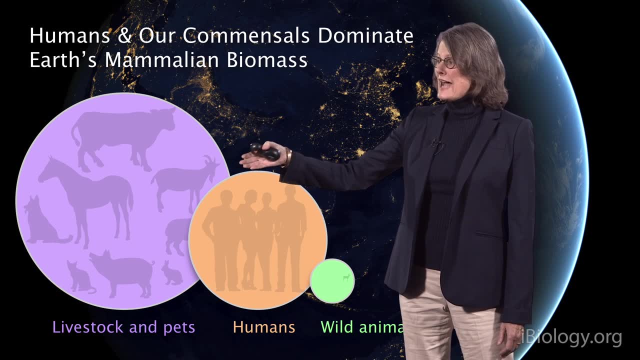 of them are threatened with death. So we're deliberately with hunting, but there's more, more than that: Humans, it turns out, and our commensal animals- cows, horses and sheep- are actually. they dominate the biomass of the planet. 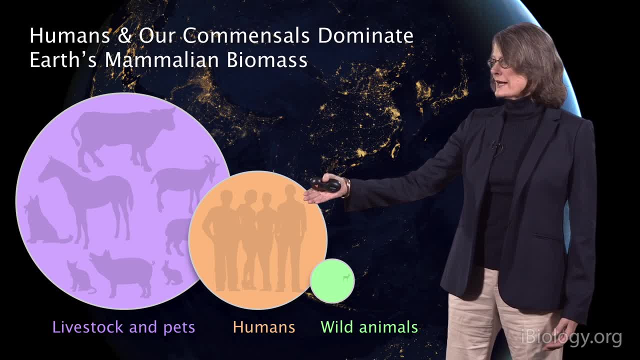 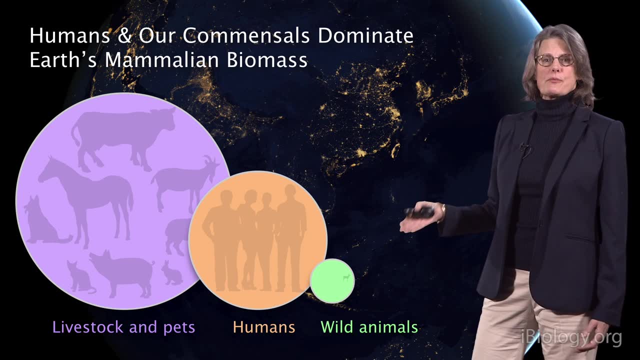 So these are to scale in terms of the number of individuals and their body mass. So you see humans here, and our livestock and pets. Wild animals, on the other hand, have just a tiny proportion of the total biomass that dominates the planet today. 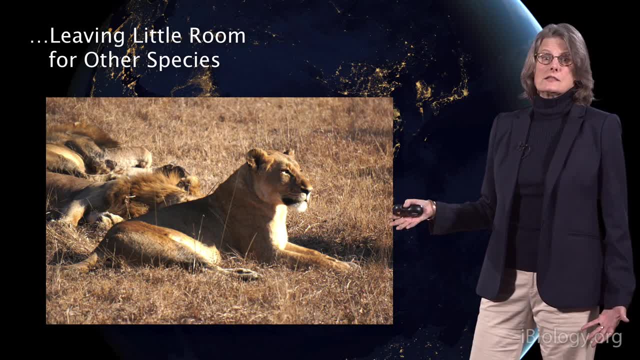 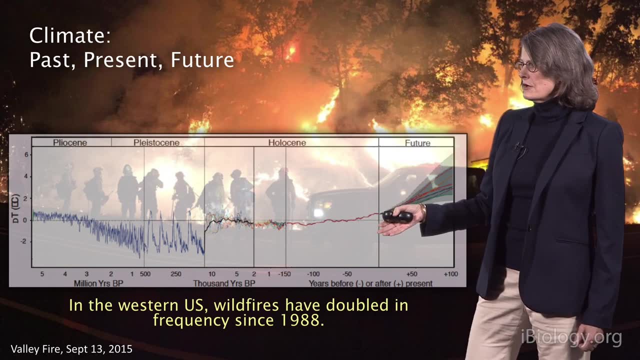 That means there's little room for these wild animals because we consume most of the energy on the planet. The other thing that's happening is climate's changing. So this is a diagram of climate change over the last 5 million years and you'll note. 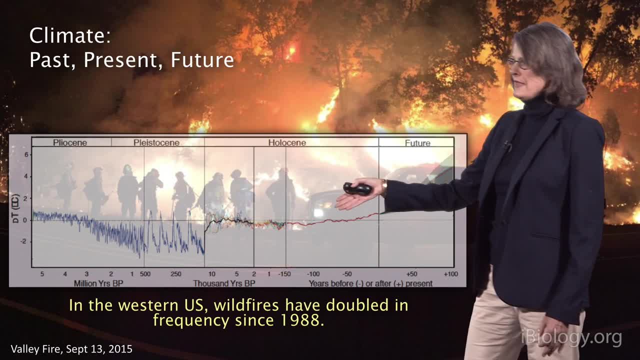 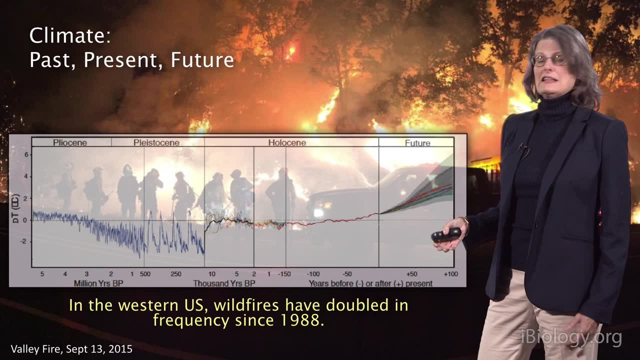 they're changing scales as we go here. It's the million years and thousands of years, and then just the number of years before present, and then we finally move into the future over here. So what you'll see is that in the last 5 million years, the climates were about ready. 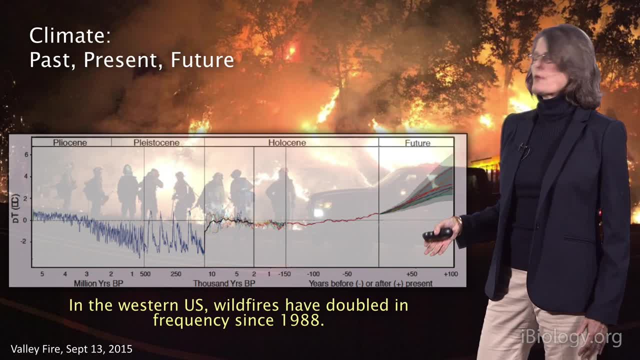 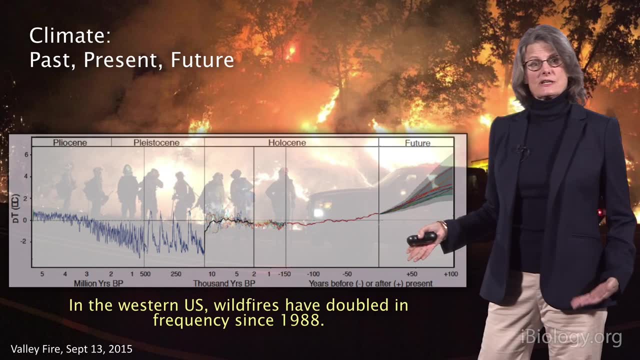 to experience within the next 50 to 100 years are warmer than anything we've experienced in our lifetime as species, and that any of the mammal species, for example, that we're used to interacting with on the planet have experienced in their lifetimes. 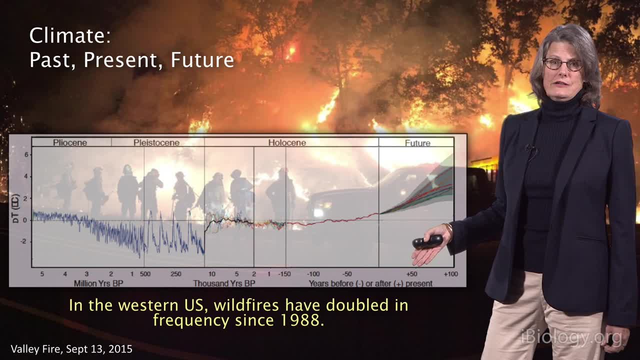 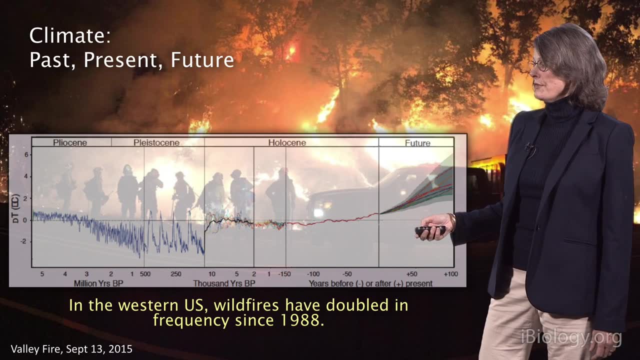 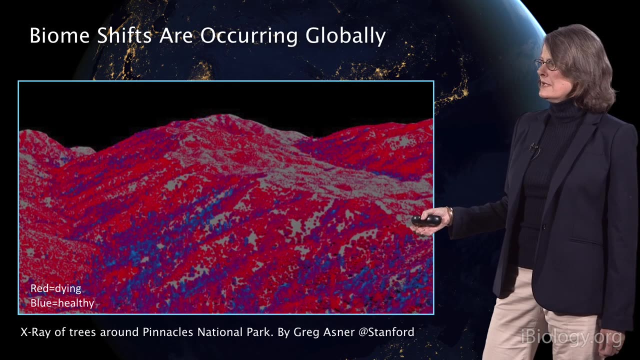 As a matter of fact, in the western US alone, wildfires have doubled in frequency since 1988, putting many people at risk for losing their homes, And that's also contributing to actual biome shifts. This is a particular X-ray image of the area around Pinnacles National Park, showing that 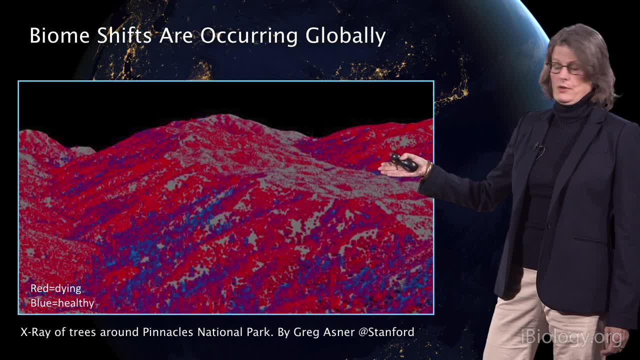 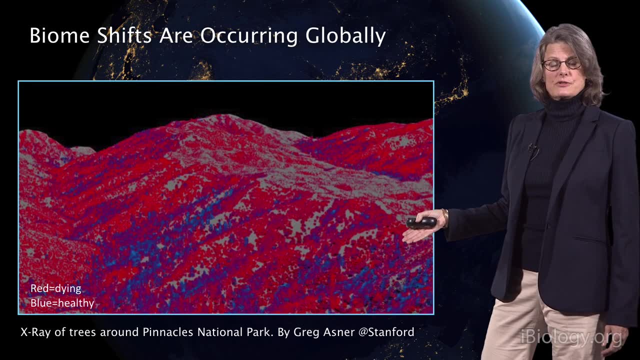 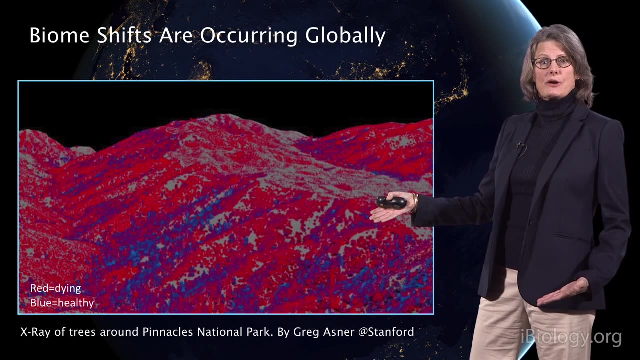 the trees that are standing there right now are threatened with death in the near future. So red, you either see dead or dying trees, and blue here are the only healthy trees in this particular environment. So in just a few years we're seeing a major shift in where trees are present and where 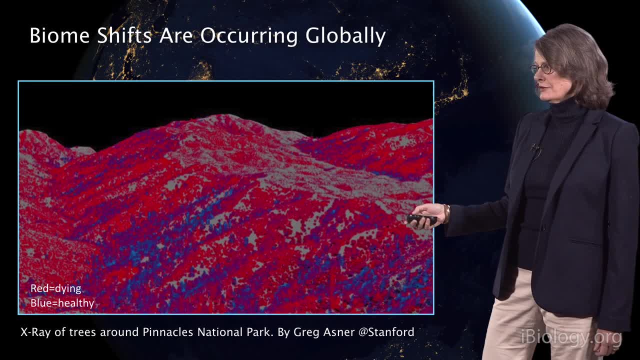 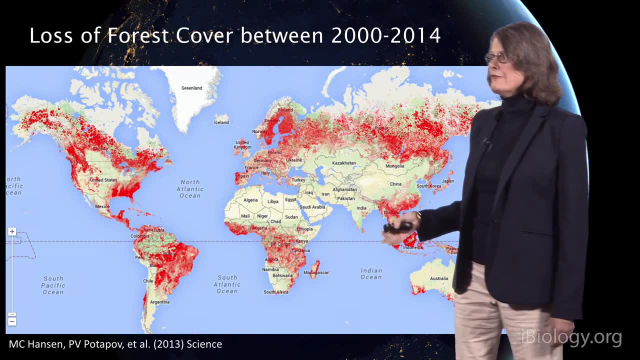 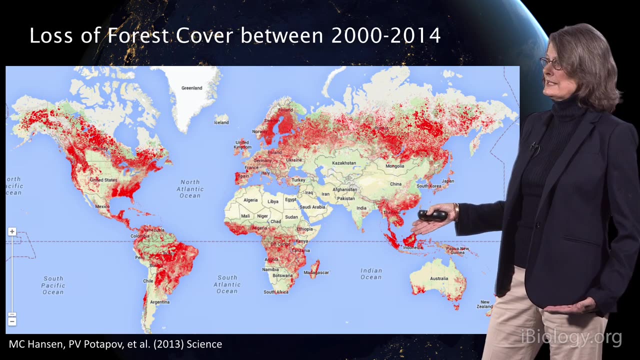 trees are not present on the landscape. That's simply because of climate and then the interaction between climate and things like beetles, in particular for trees. We've lost a tremendous amount of forest cover. The rate of loss has slowed down, but that doesn't. that really doesn't matter in some. 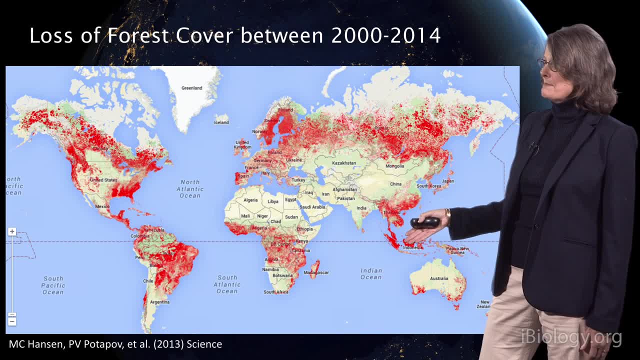 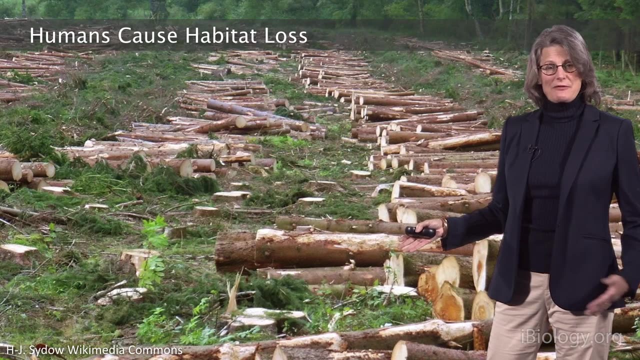 ways, because we've lost a very, a vast amount of many of these forests in in just the last 14 years around the world. Humans, in fact, are really good at causing habitat loss. We can just basically go out. this is like hunting for trees: we go out and we are. 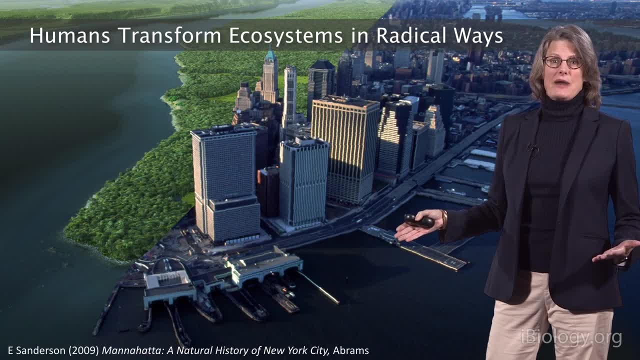 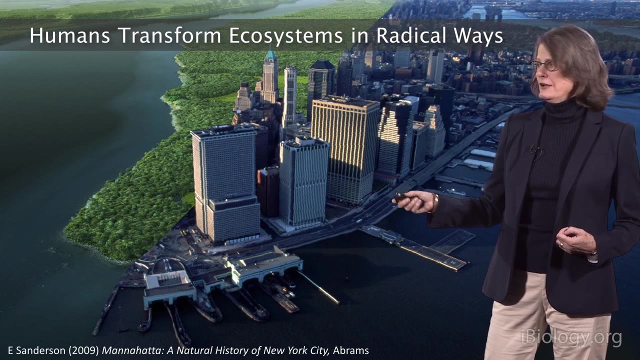 just take them down, We transform ecosystems in radical ways. This is an image of what New York used to look like before we actually built up this city next to what the place looks like now, And clearly there's no way for biodiversity- at least most biodiversity- to thrive in an 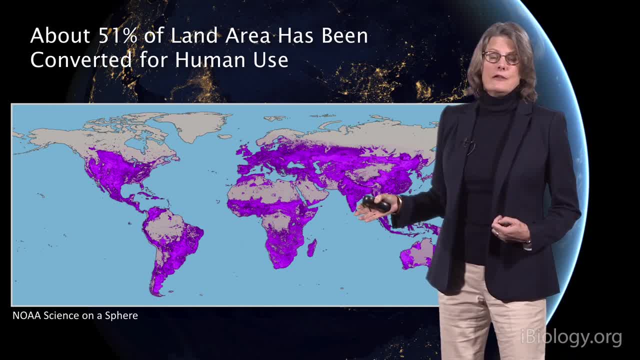 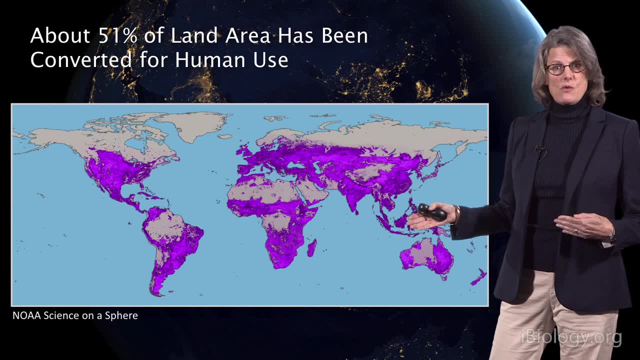 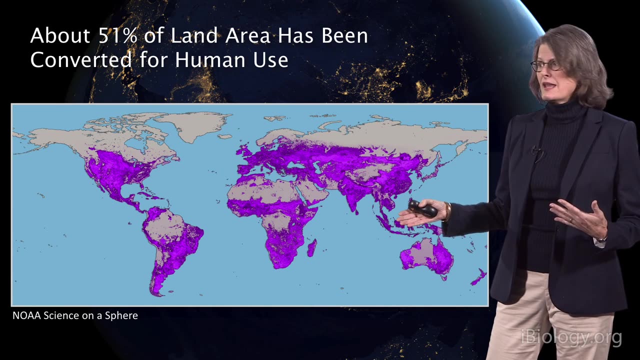 environment that's so human-dominated. In fact, if you look at the sum total of the terrestrial land on the planet, we have used and co-opted about 51% of the land area just for our use, mostly for production of food for ourselves and our commensal animals. 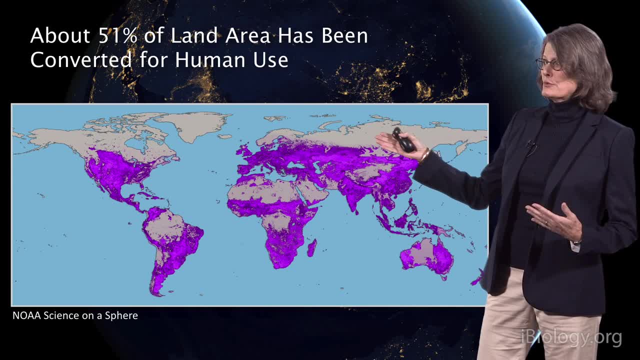 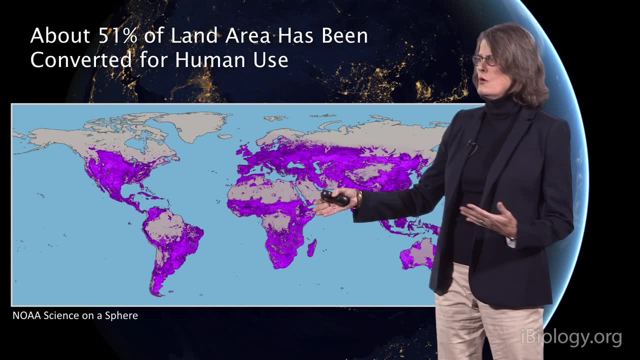 If you look at this, you'll see that the only places that we haven't really occupied and we haven't transformed are the hard-to-reach places: the Sahara Desert, the Congo, the Amazon, two of the places that have the most 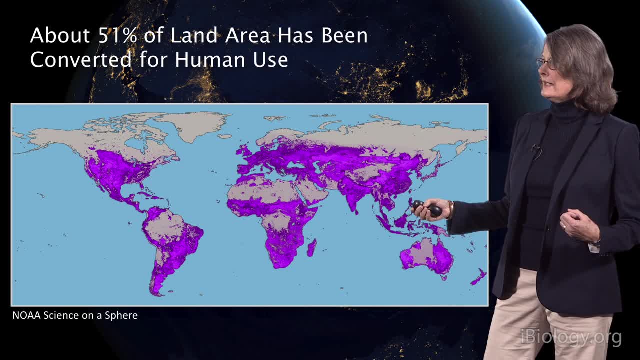 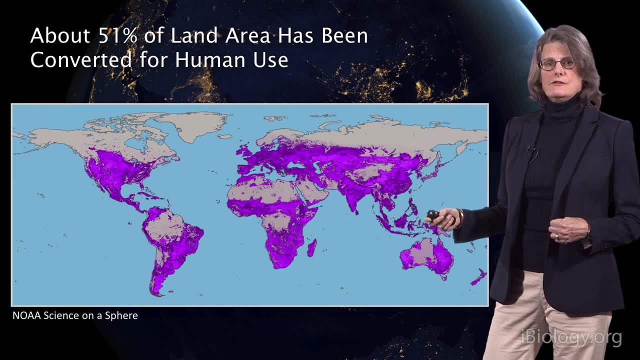 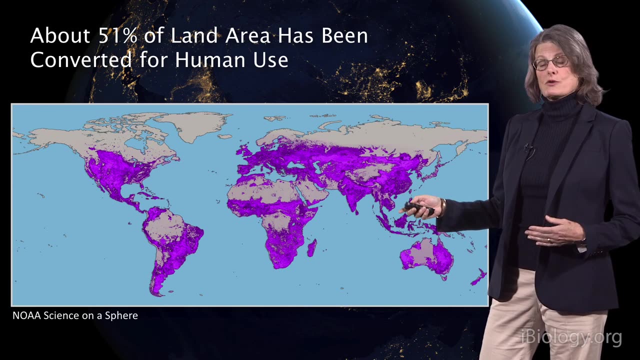 the largest, you know, tropical forests left in the planet and the boreal forests and the tundra region. So we've taken all the easily farmable land in the world. Now we need to basically farm this land we already have co-opted more efficiently in. 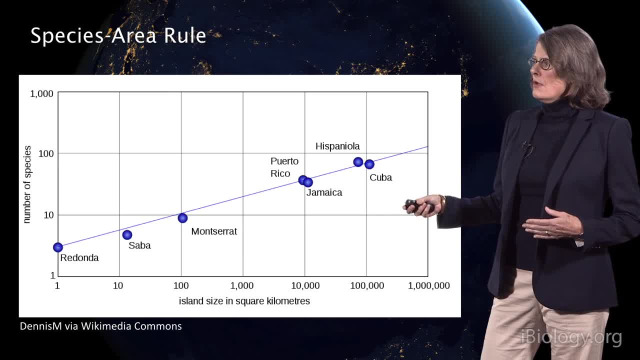 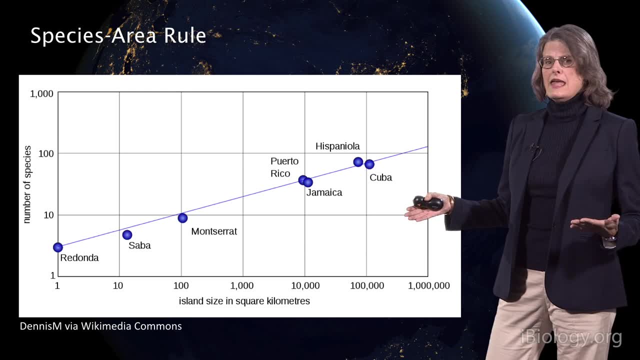 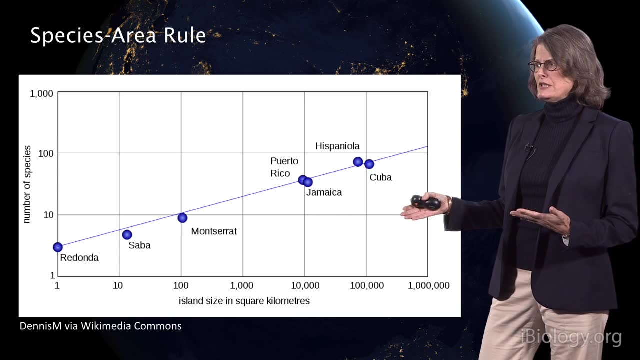 order to feed the coming mouths. One of the things that matters a lot when you think about how much of the land we've actually changed on the planet, is that just by this simple rule. one of the fundamental rules in ecology is that the number of species is a function of 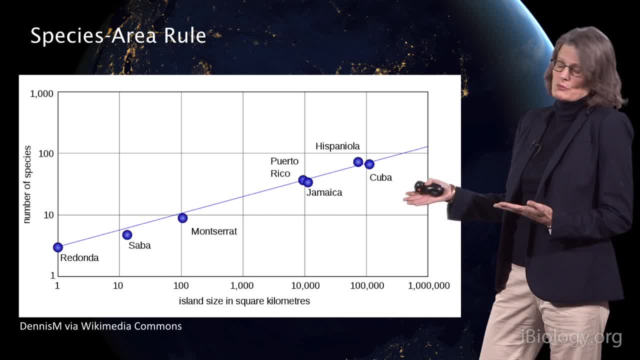 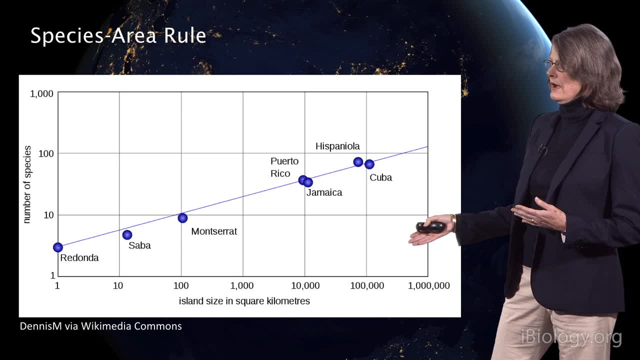 the size of the place they occupy. This is a rule of island biogeography, And so here, what we see across the x-axis is the size of the island- these are islands in the Caribbean- and the number of species on the y-axis. 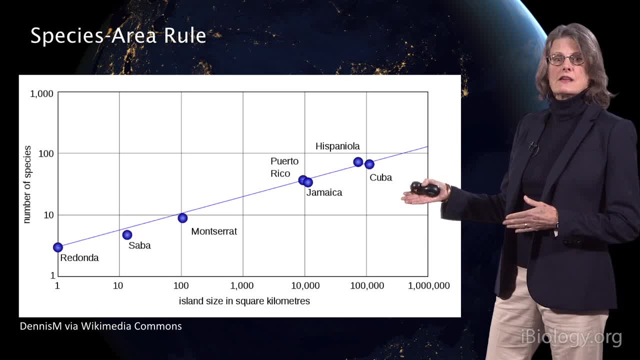 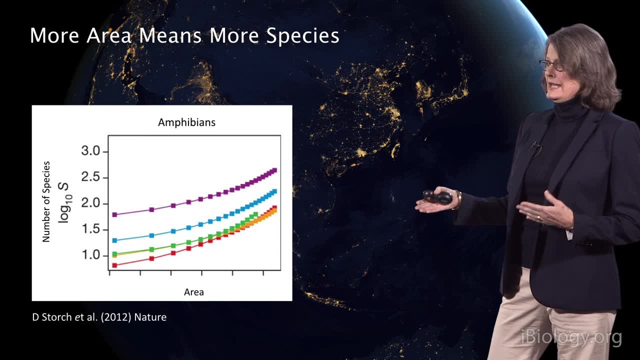 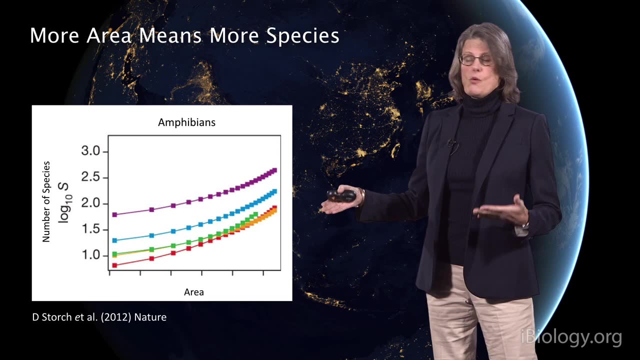 And so the larger the island is, the more species are found on the island. More area means more species. Here you see an image for different continents on the planet and the number of amphibians. So even on a continental scale we're finding that larger areas mean more species. 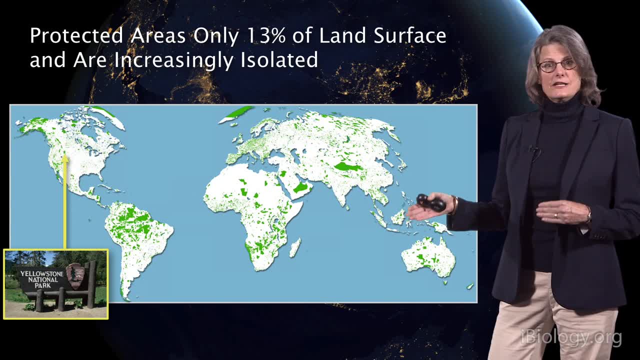 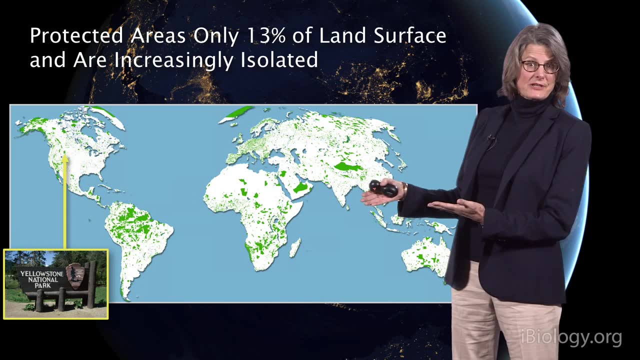 So when you look at the amount of land we've actually set aside to be protected on the planet, it amounts to only 13% of our land surface. So even though we've co-opted the function of 51%, we've only actively set aside 13%. 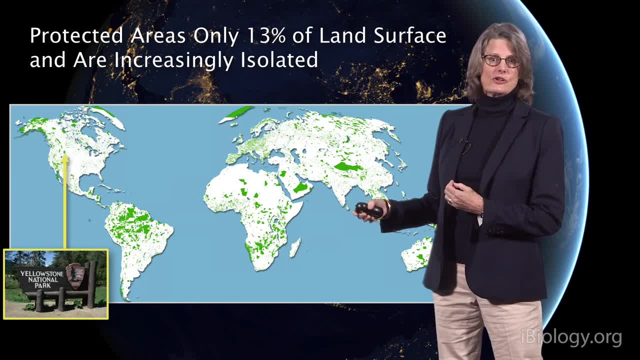 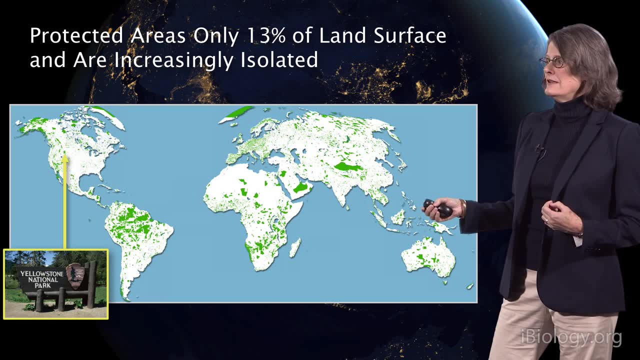 of this to be protected, And areas like Yellowstone National Park, the world's first national park, as you can see, isolated from all the other protected areas in North America. So what these patches mean is that we don't have a lot of connectivity between our protected areas. 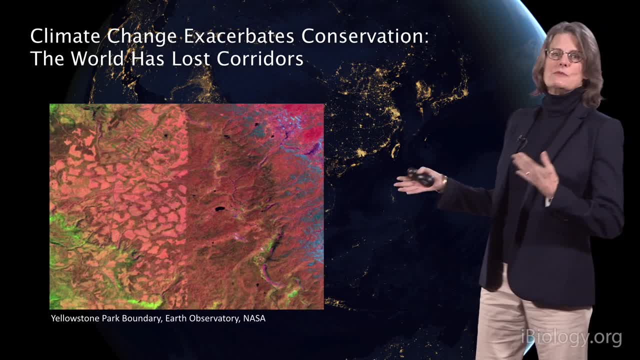 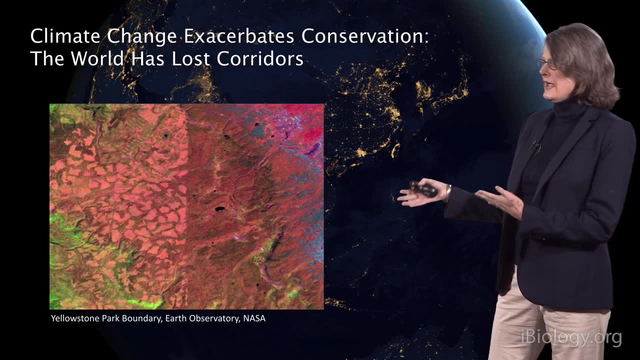 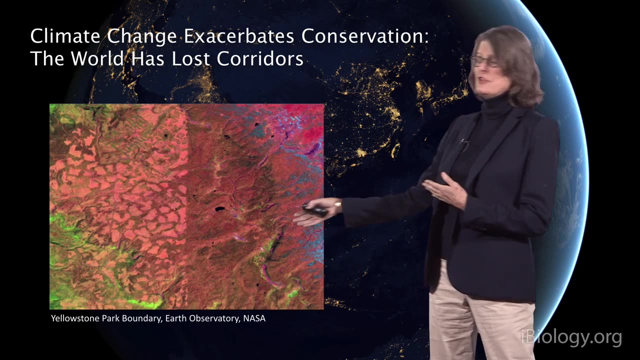 That exacerbates our attempts at conservation, because animals like to move to deal with different environments. as the climates change, They like to move to novel environments. This is Yellowstone National Park seen from Earth Observatory, And what you see is a very is a nice long line there, showing you the division between: 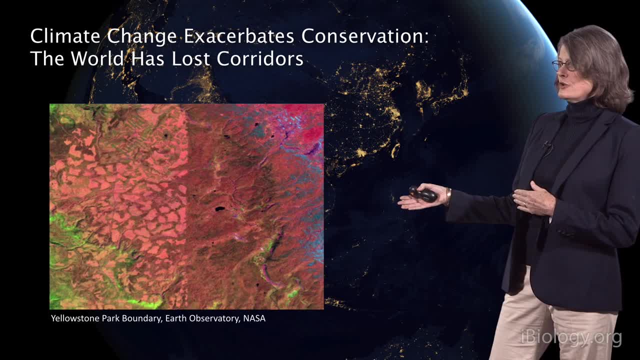 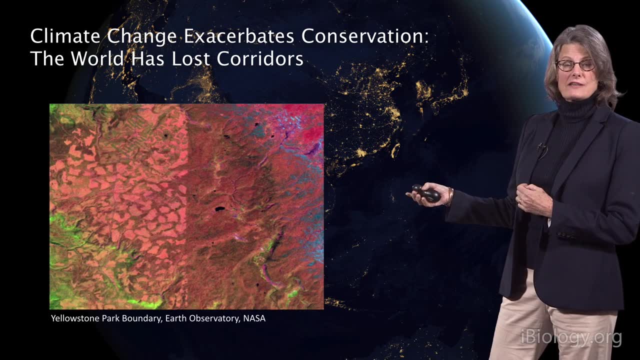 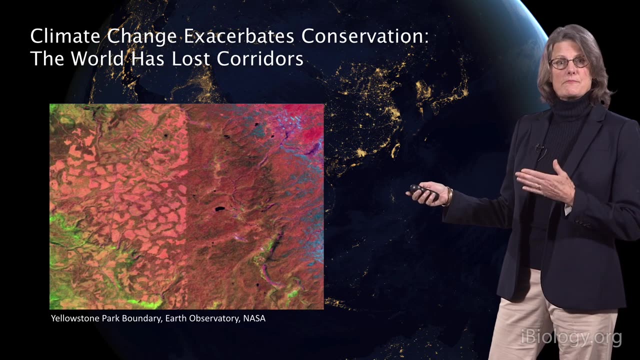 the Forest Service land on the west and National Park land on the east, And what you'll see is clear-cutting defines now the western border of Yellowstone National Park. This is true for many of the protected areas in the world. There's not a lot of buffer. 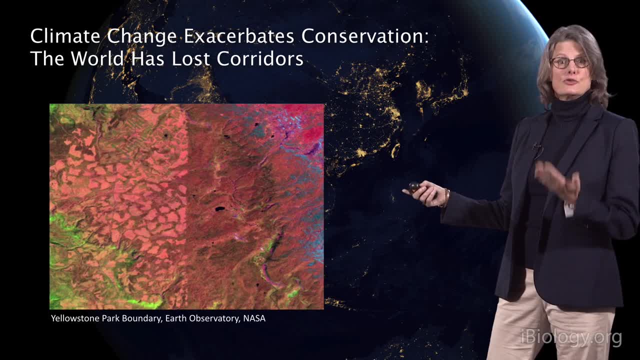 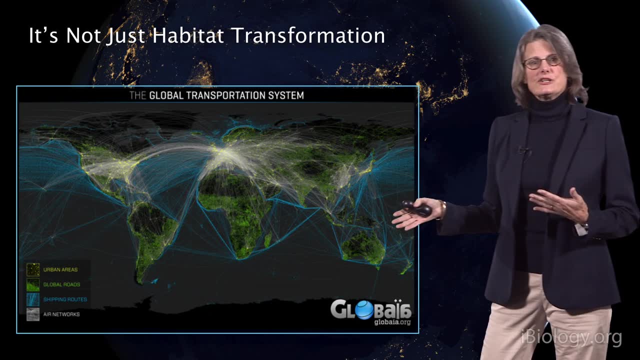 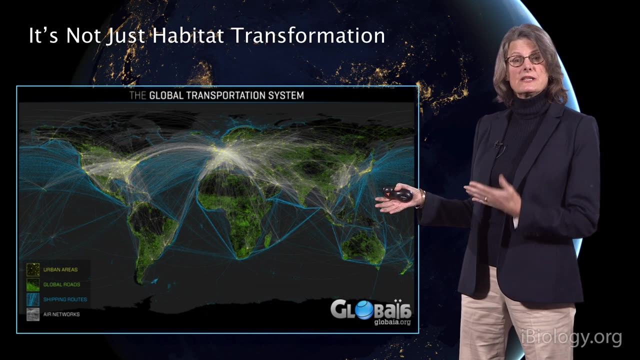 And this is true for the animals that want to move away from Yellowstone to a part of the landscape that they can adjust to. It's not just the transformation of habitat that matters either. It's that our transportation system itself has disrupted a lot of these corridors of connection. 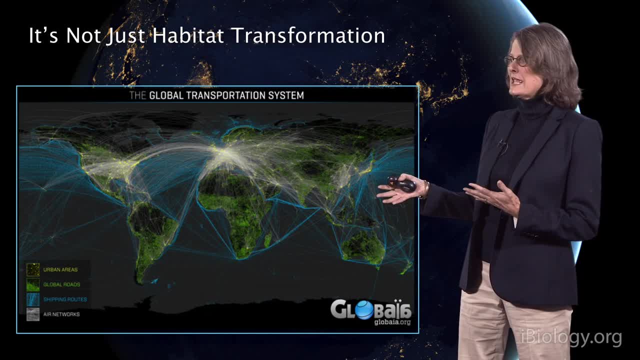 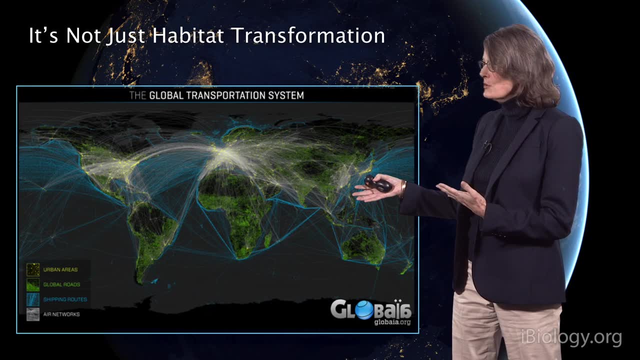 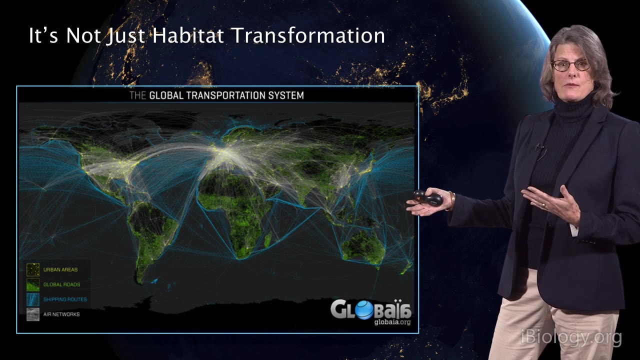 This slide, which is really spectacular at showing how much of the landscape we've cut up with our transportation, shows that in green you see in the global roads, you see in yellow our urban areas, in blue you see our shipping routes and in white you see our air networks. 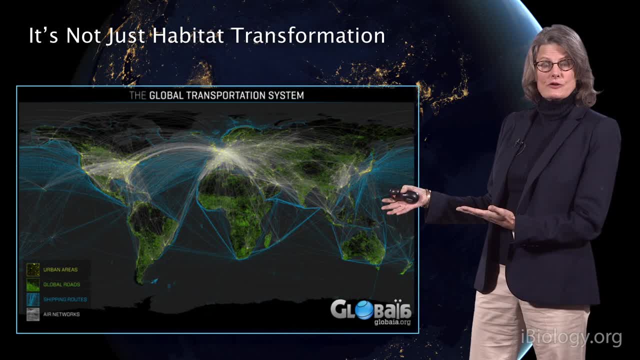 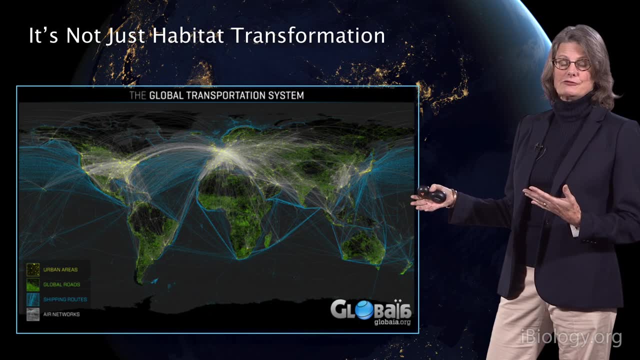 So it's not just on land, It's not just what we've kind of transformed in terms of deforestation, It's the roads we've built, it's the number of ships we send across the ocean and it's the number of planes that fly in the sky, all of which interrupt and threaten animals. 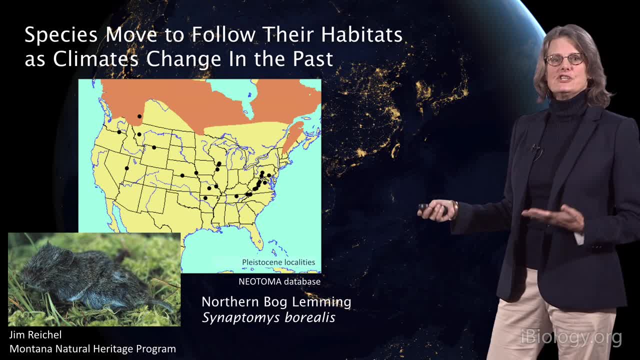 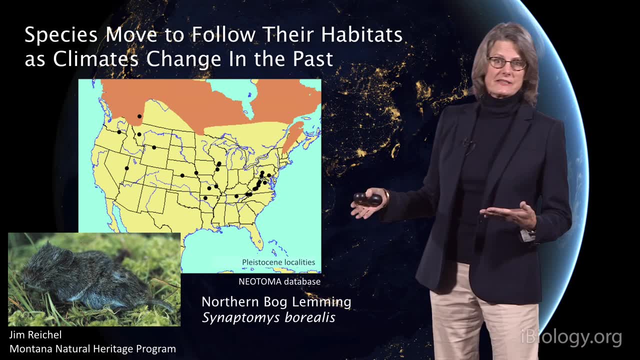 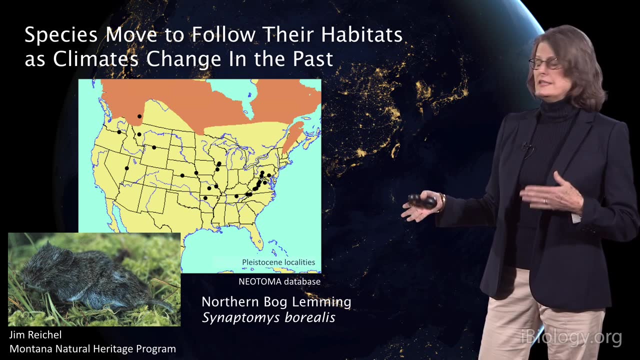 that need to move across this landscape. These species move to follow their habitats and they've done this in the past. This is, in fact, one of the first signs of adjusting to climate that we see On the black dots. here you see our data from the Pleistocene showing that these animals 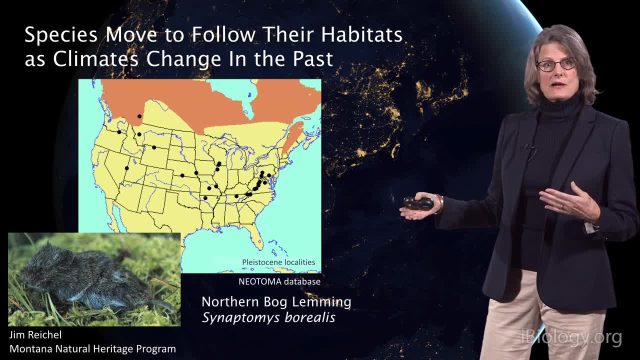 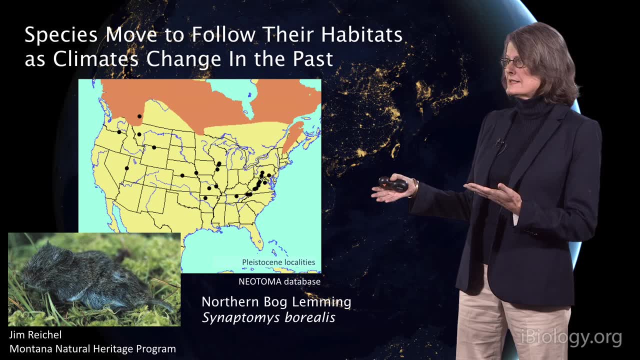 used to be present greater than 10,000 years ago, somewhere between 10 and 20,000 years ago, at these parts of North America, And as climates warmed at the end of the Pleistocene into what we call the Holocene, which is the 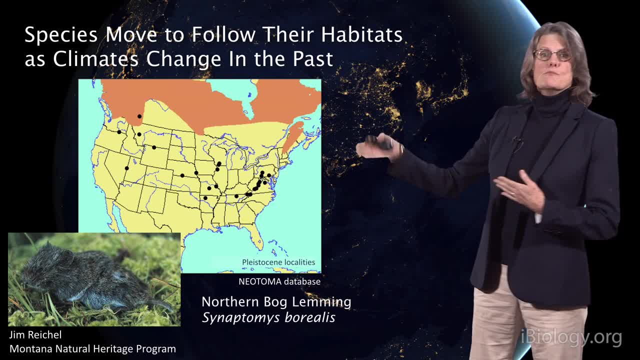 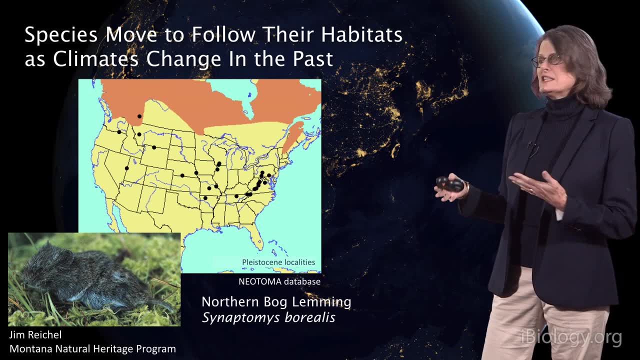 last 10,000 years. this species- this is where bog lemmings moved to the north and now you see its range is occupying the orange part of this figure. So these species just responded by moving poleward as climates change. 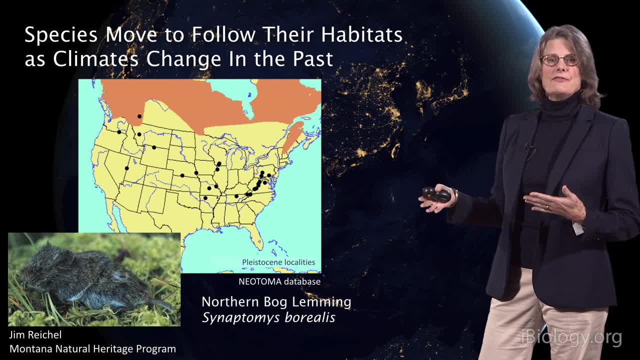 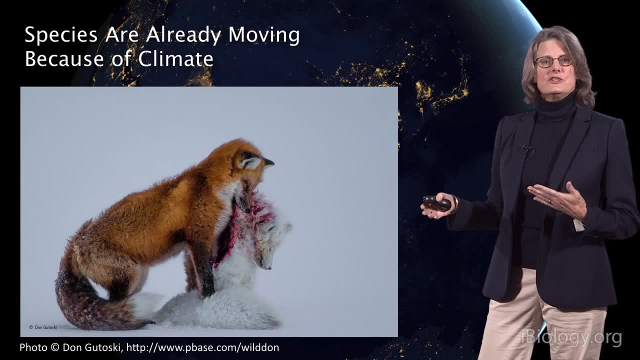 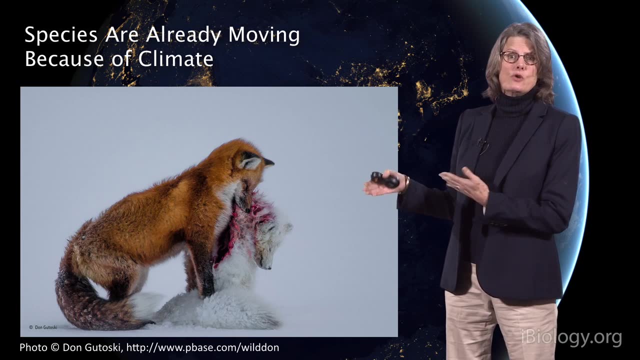 This is a very typical response among animals of the world: that they move poleward as climates warm and they move equatorward as climates cool. In fact, species are already moving north today. These are examples of species interacting with species that don't they don't normally see. So southern species are now starting to encounter species from northern boreal forest or tundra regions and there are really interesting and sometimes not very positive interactions that result from those interactions. They create new ecosystems. So these are animals just doing what they need to do and challenging us too in thinking. 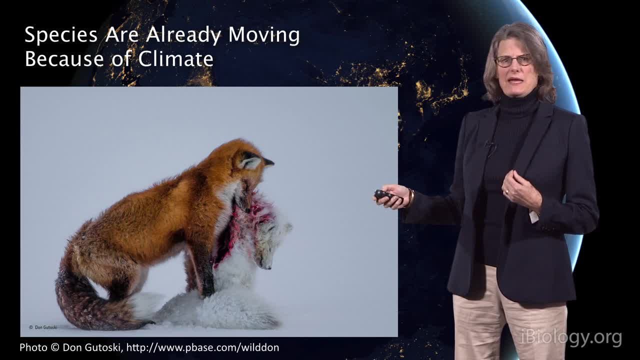 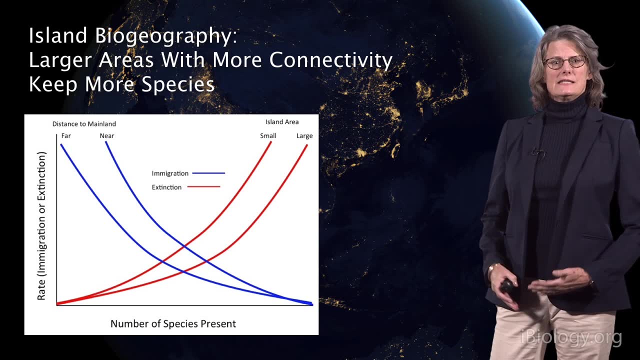 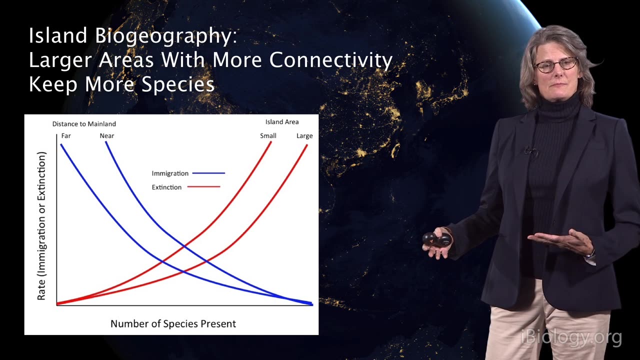 about what natural, what pristine, what we should expect in the future. So I already said that animals are on the move and what that means is that they need to find areas that they can colonize, where they can live, And it turns out that this fundamental rule of island biogeography- that includes more. 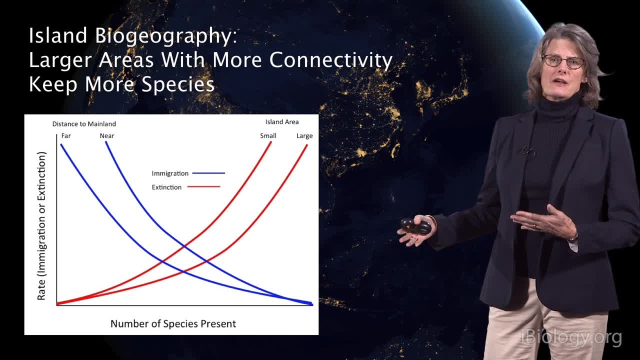 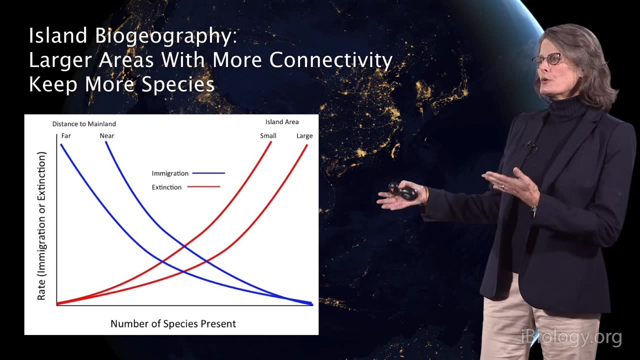 larger area means larger number of species. it also includes a concept of connectivity, So the closer these islands or these populations are to each other, the more likely they are to maintain more species. So what you see across the x-axis is the number of species present and this is the 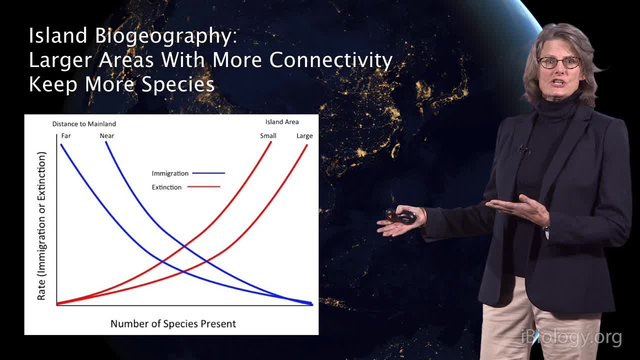 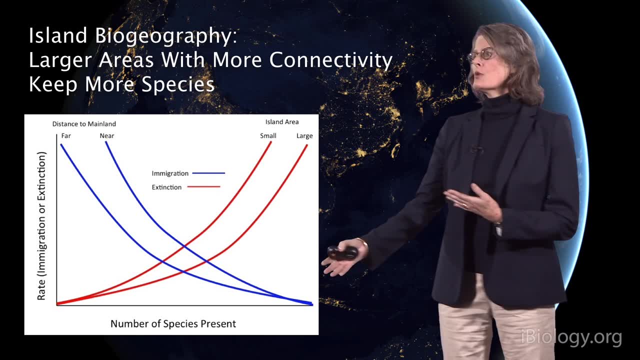 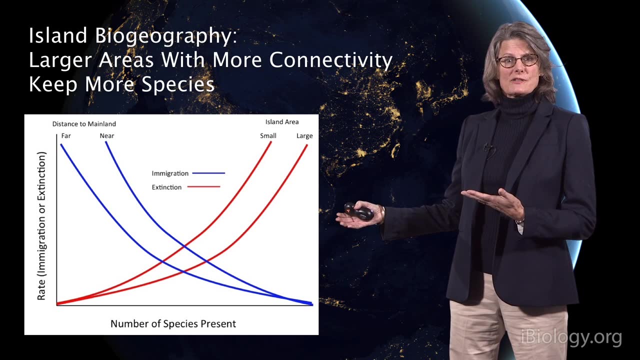 rate of extinction, shown in red, and immigration, shown in blue. And so when the when the populations are far from the mainland, there are many fewer species that can be maintained, and when they're close to another population, they can maintain more species. 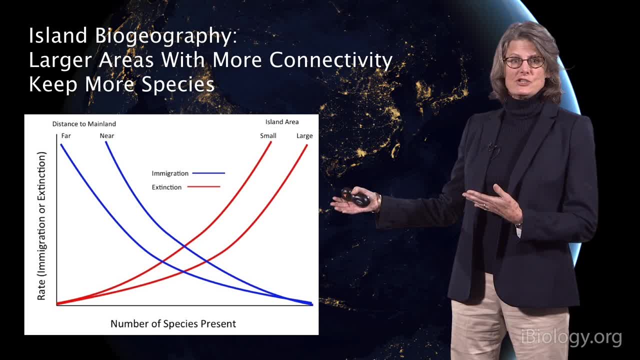 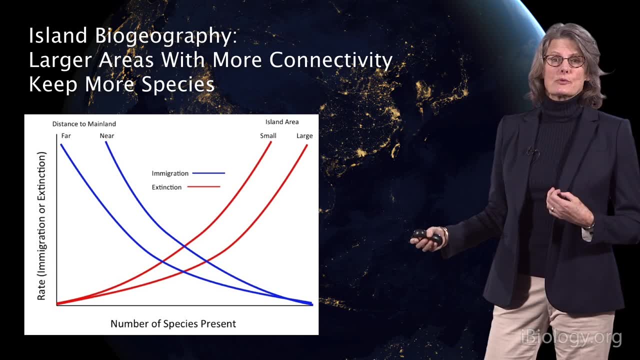 Likewise, when the island area is small, it maintains very few species compared to when the islands are large. So it's this equilibrium, it's this balance between these rates that really matters, And we have to think about this in moving into the future. 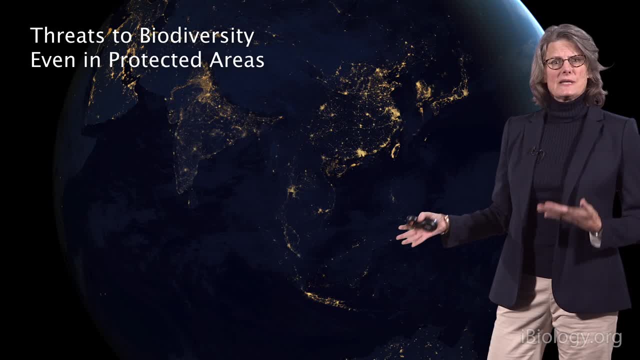 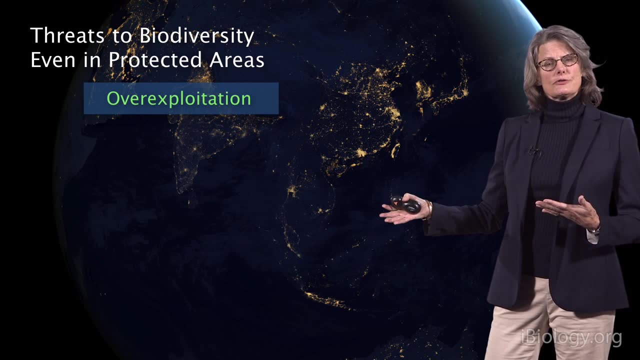 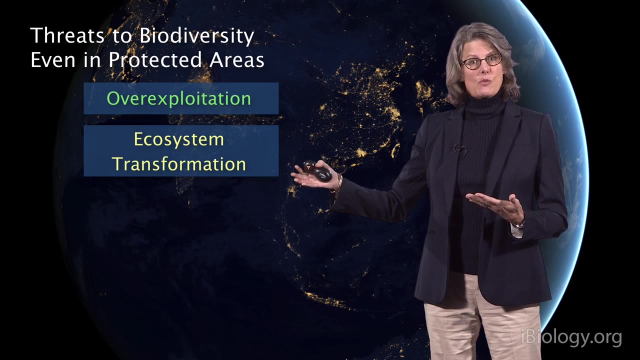 So really, what that means is biodiversity is threatened, even in protected areas, And it's threatened surely by overexploitation, by hunting, deliberate poaching, But it is also threatened by ecosystem transformation. Protected areas don't preserve entire ecosystems, and so the transformation of what's happening. 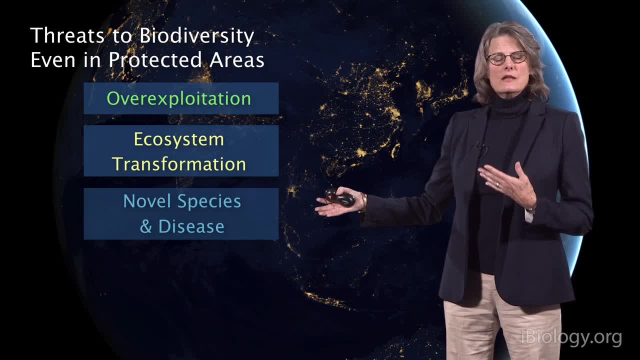 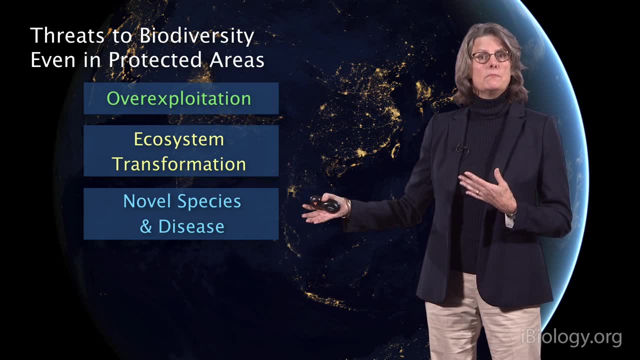 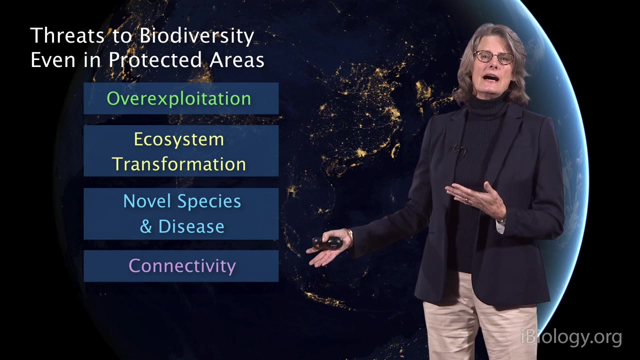 in protected areas matters to the species that live within it. Novel species are interacting with disease and bringing new diseases into places they haven't yet been, because they're responding to climate change and other sources of environmental transformation, And that means that connectivity between these protected areas is very important. 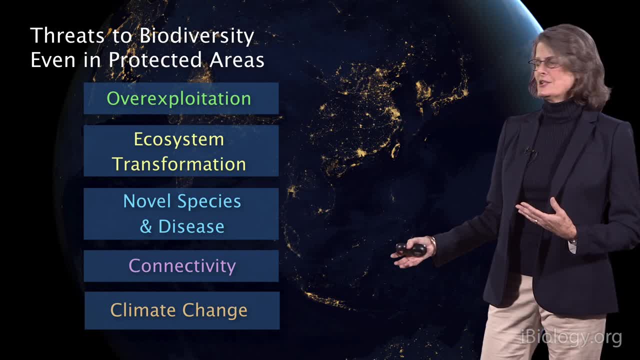 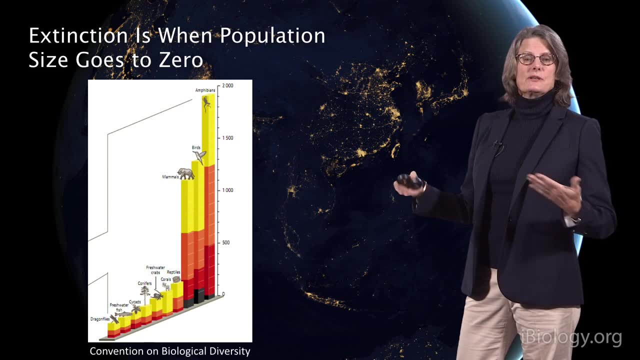 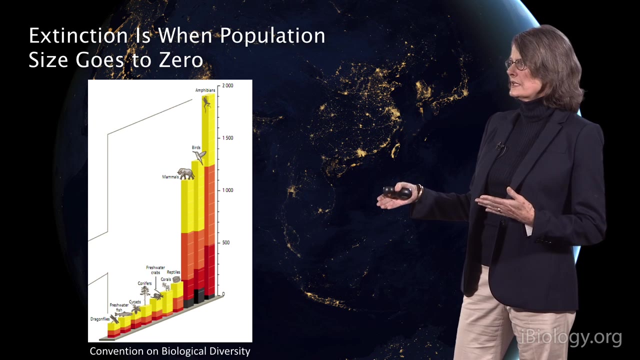 So, finally, the thing that's really pushing all of this is climate change, and that's what's very important to consider going into the future. Now, one of the things that happens as populations get fragmented is that their population size, the animals' population size, starts to decline. 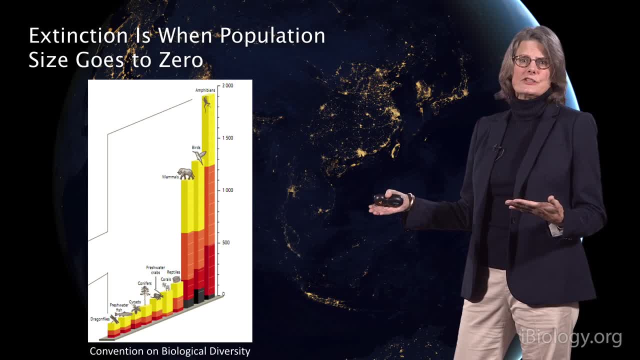 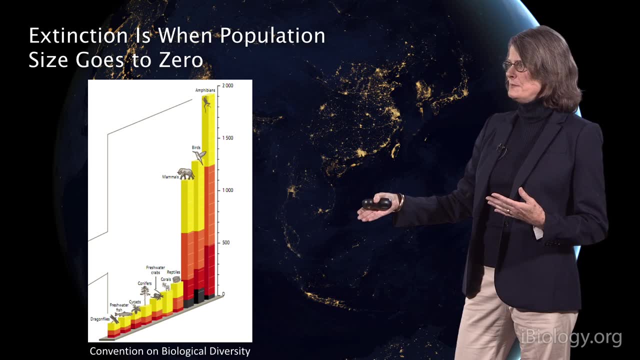 And extinction. the loss of a species forever on the planet- is just when population size goes to zero. So here we see amphibians, birds, mammals and other many other species, and these are all animals that are threatened somehow with extinction. 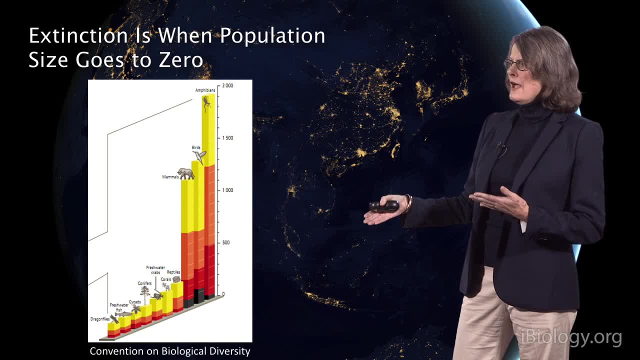 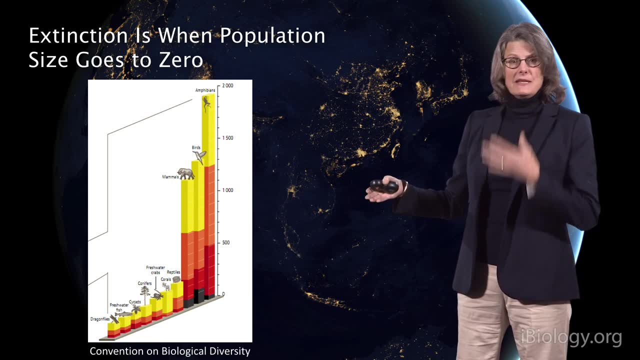 There are animals shown in black that are completely extinct in the wild. There are animals that are shown in these, in these warmer colors, that show different kinds of threats to their systems, whether they're imminent- they're facing imminent extinction, or whether their populations are threatened. 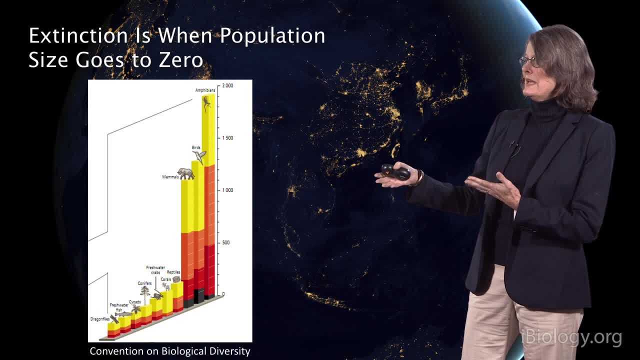 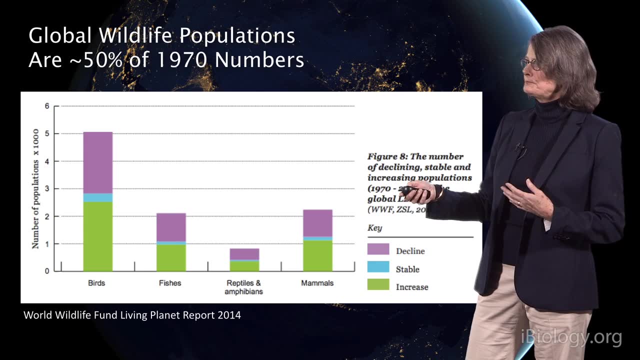 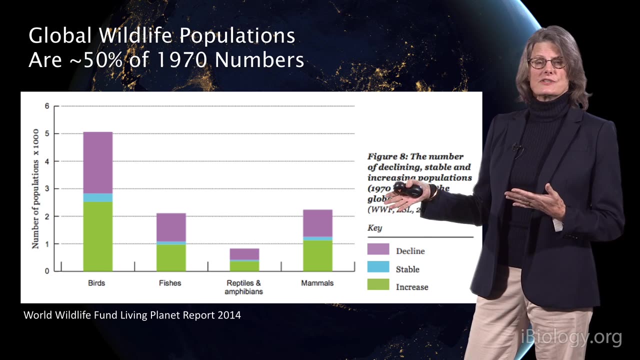 And so all this is to show is that there are many animals, many, over, you know, thousands of animals- that are threatened with extinction because of population demise. In fact, global population numbers of wildlife are 50% of what they were in 1970.. 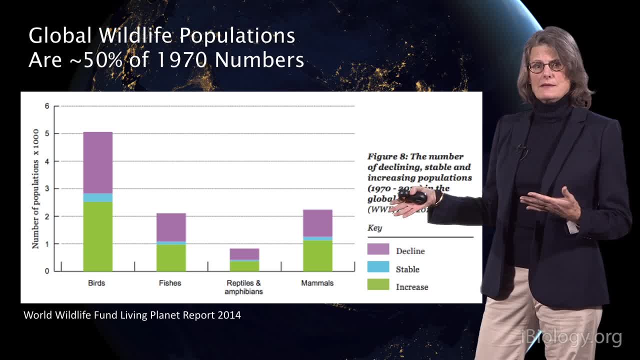 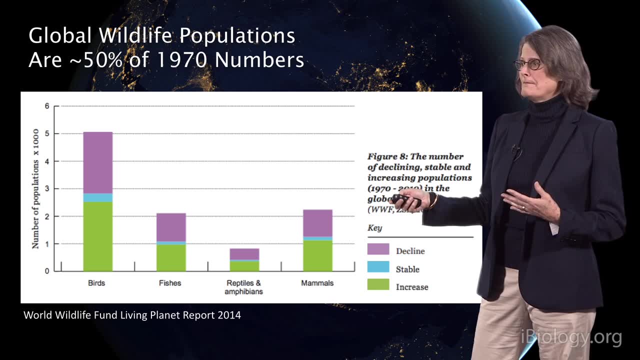 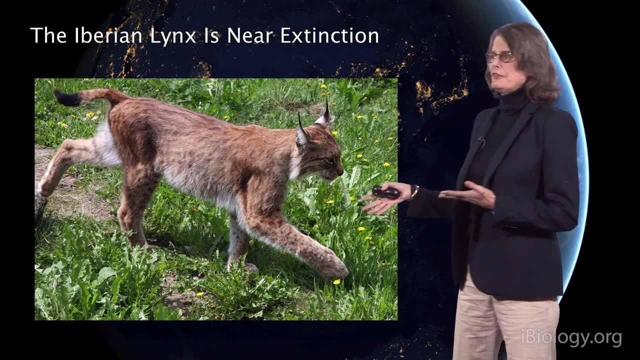 So animals of all types- birds, fish, reptiles and mammals- are showing really large declines in the number of populations that are on the planet. Just the number of individuals of these species is declined by half. I want to give you an example of what this means. 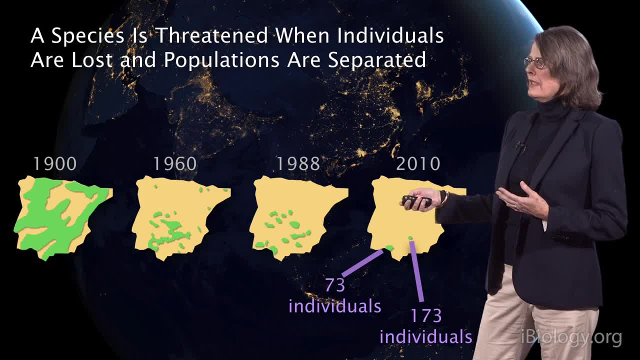 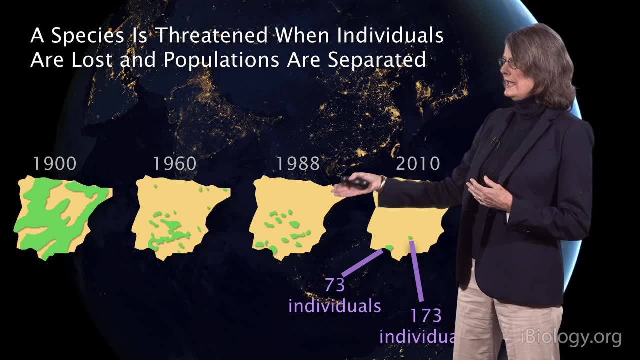 So this is the Iberian lynx. It's found in Spain And this animal, in 1900, was occupied most of Spain And you can see its demise. So in the 70s, the 80s and in in 2010, there's, there are two populations remaining. 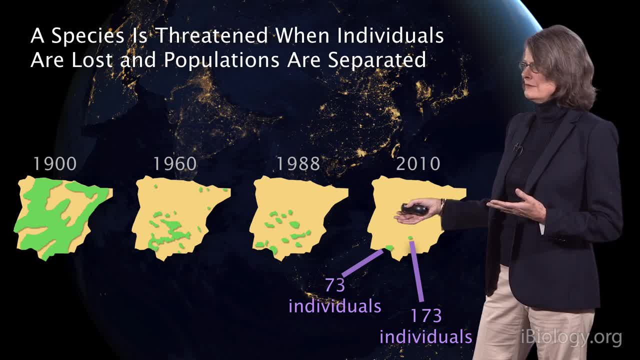 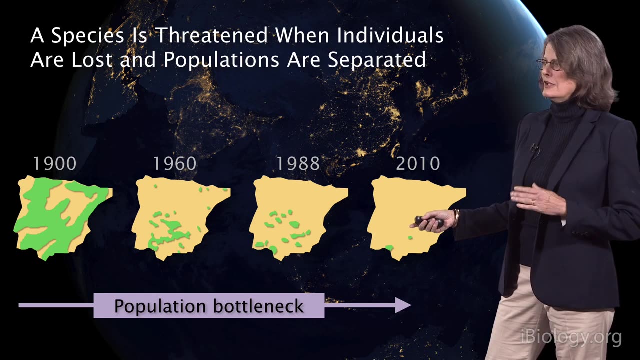 one with 73 individuals and the other with 173 animals, individuals. So not only have we lost populations, and clearly we've lost individuals, we're just down to a couple hundred of these lynx. And what does that mean? It means that they've gone through what we call a population bottleneck, and I'll explain. 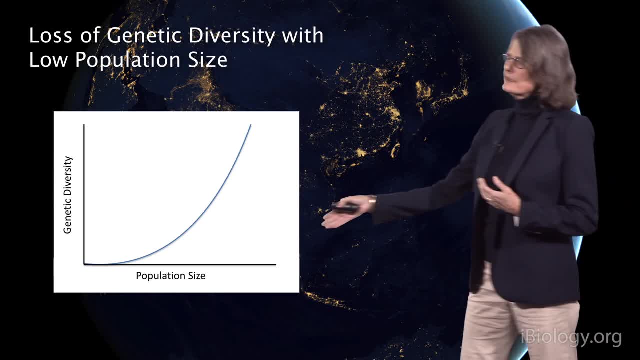 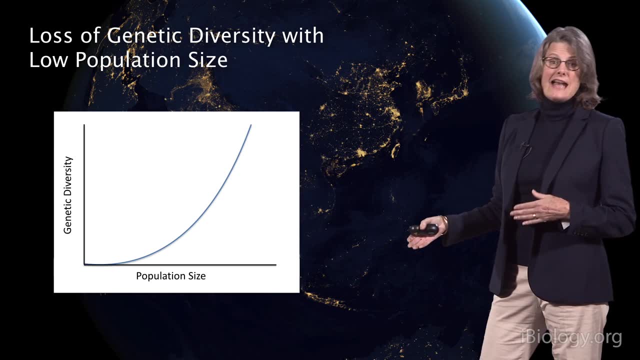 what that means to the species in just a second. So what we see is that as population size declines, so as we decrease population size, we actually decrease genetic diversity as well, And so, in general, the larger the population is, the more genetic diversity will be maintained. 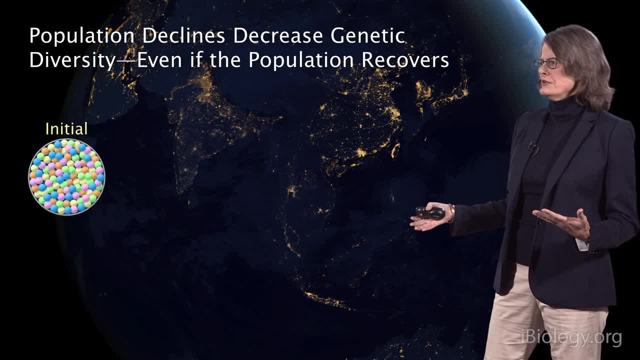 in that population. And and why do we care about population diversity? We care about population diversity because that's the toolkit that species have to move into the future. So if we, you know, we have a little simulated model here. 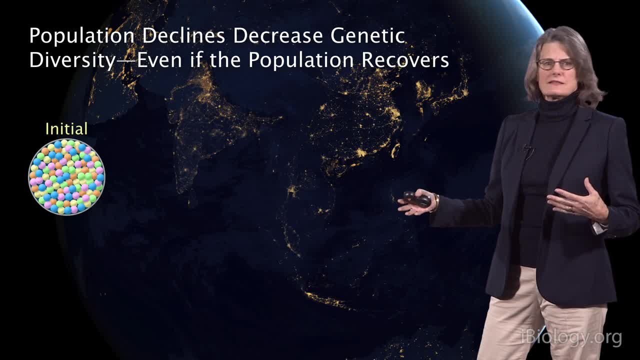 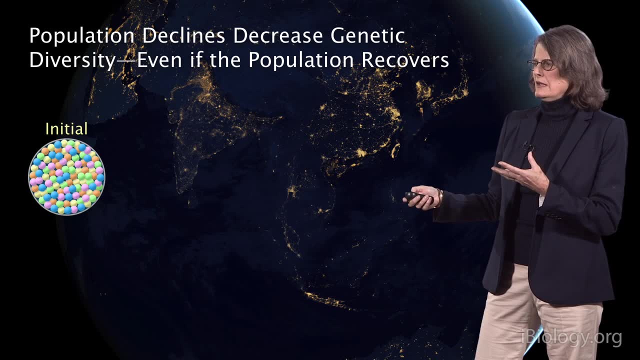 If you think of every one of these marbles, these different colored marbles, marbles as some sort of a genetic diverse, different kinds of a genotype of some sort, if we start with a lot of genetic diversity and then you just grab a few of these marbles, you're gonna get a bottleneck. 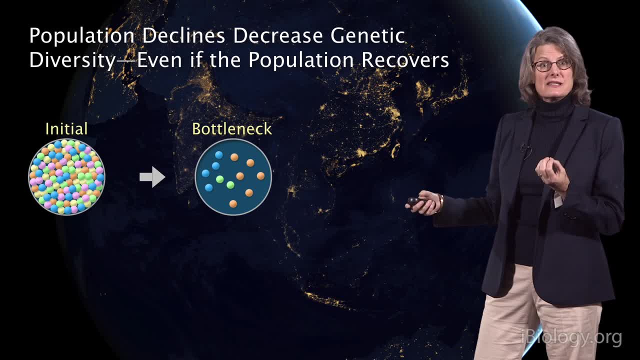 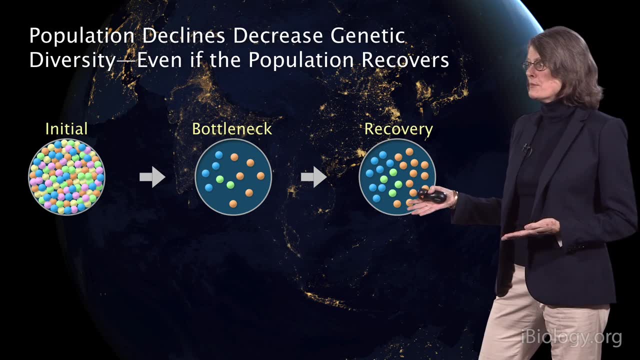 There's no way you can get all of this diversity. if you decrease the number of marbles you've pulled out of the system, That's called a bottleneck, You can recover. You can recover in numbers. You can actually start reproduction of this, of this particular hypothetical species. but 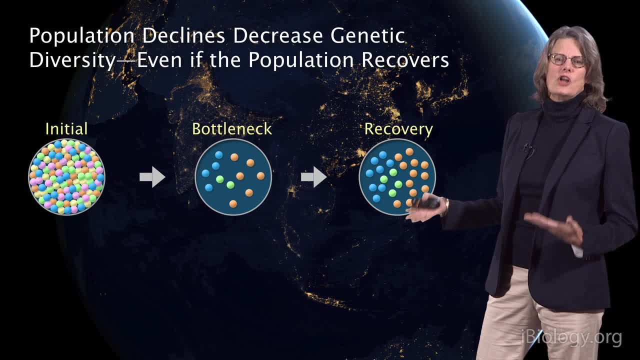 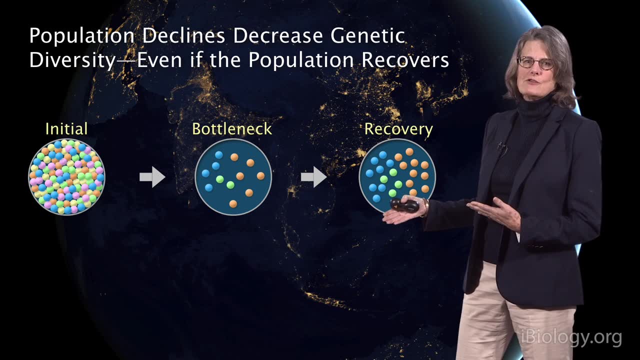 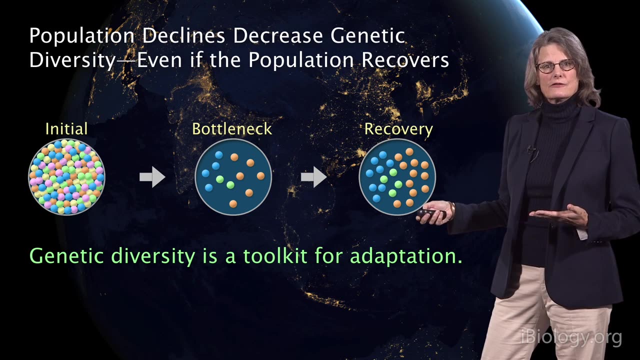 you can't recover the initial genetic diversity because it takes so long in evolutionary time to accumulate. So not only are numbers of individuals important, it's important to retain those individuals as long as possible to maintain genetic diversity. Genetic diversity is a toolkit for adaptation. 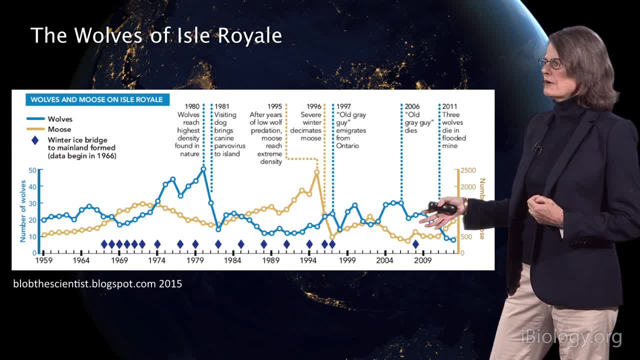 Here's a great example. These are the wolves of Isle Royale. They're they've been studied for over 50 years. It's the longest study of a predator-prey system that we know about. Wolves colonized this island in Lake Superior in the 1940s and they bounced around. 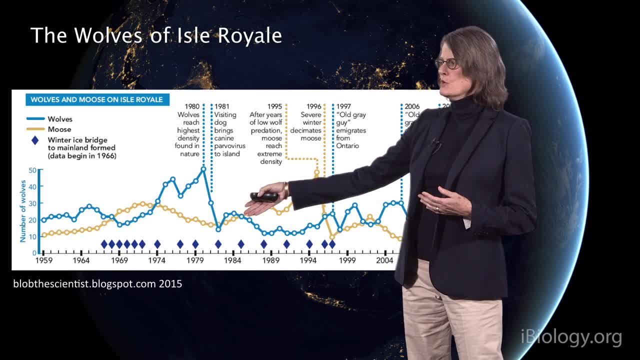 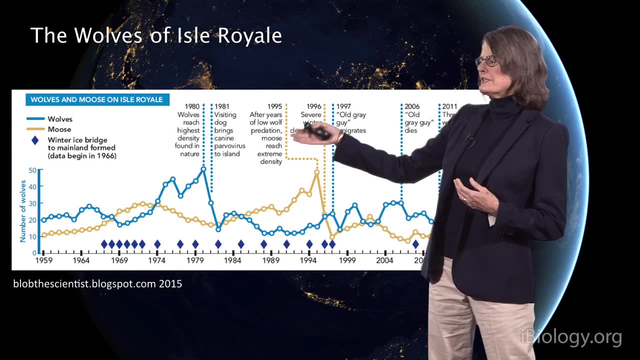 There's a pretty close relationship between wolves and their moose prey, where there there's kind of a dynamic between the two of them. They've there's been some severe winter declines in moose and then that affects the wolves in some way. 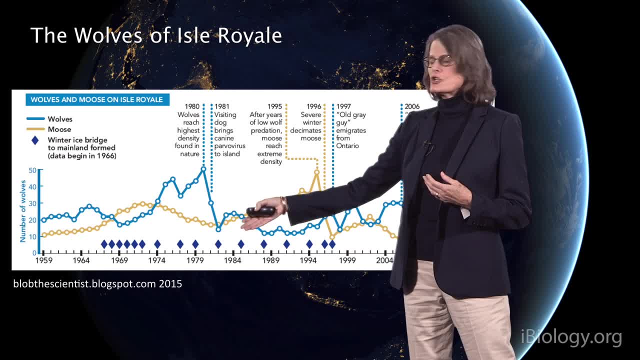 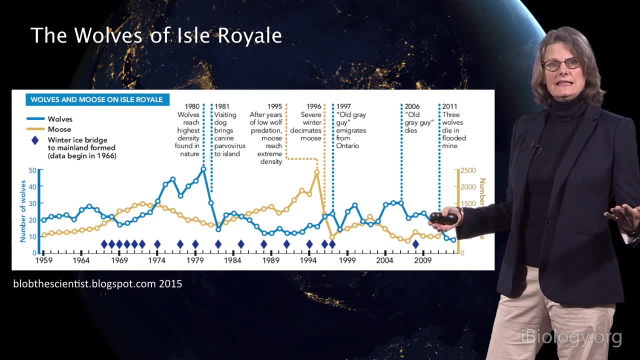 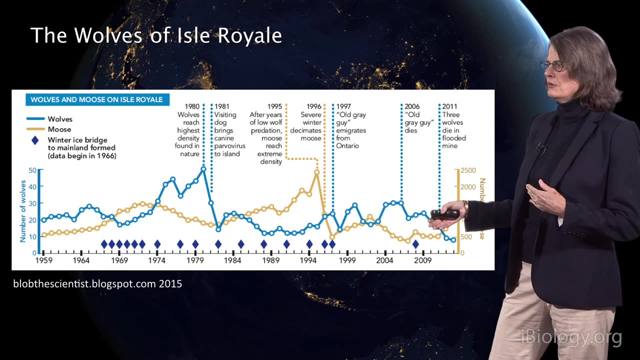 There's also been a particular canine parvovirus that caused a large crash in the number of wolves, and every one of these diamonds shows you that there was a winter bridge to the mainland that wolves could colonize across, And so they, it's contin. the population was continually being rescued. 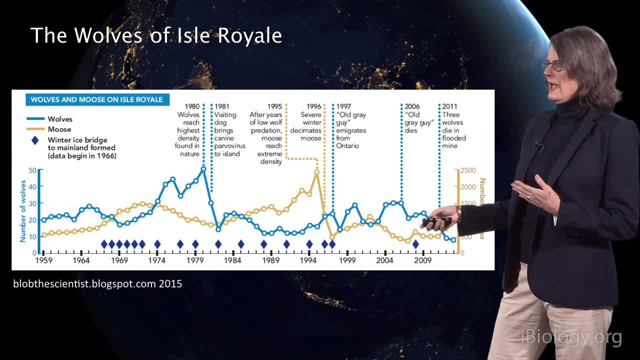 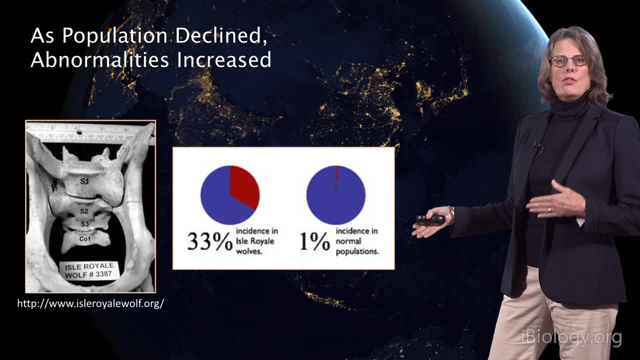 You see now that that there aren't very many of these colonization events and and in fact the wolves are in decline, And in decline because they're they, they're losing their genetic diversity. abnormalities in this population have increased dramatically. 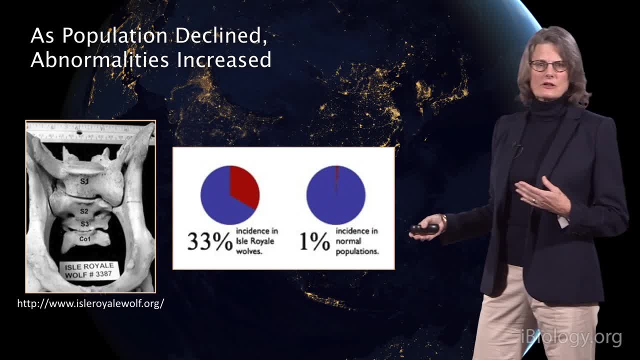 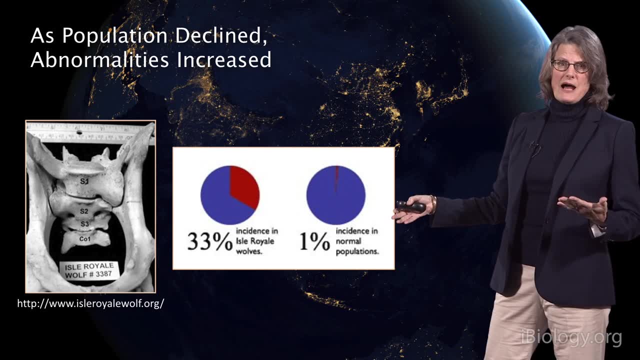 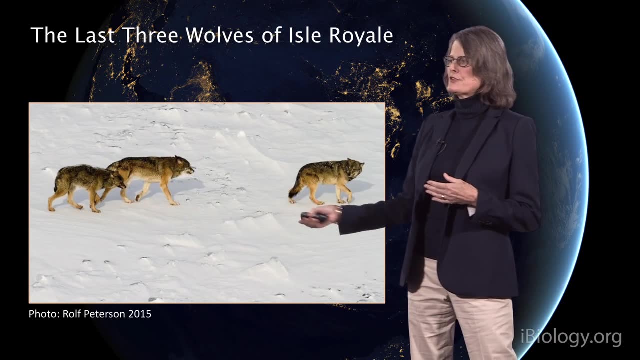 So, for example, these particular abnormalities in their spinal column in in Isle Royale, their incidence is about one in every three And in a normal population it would just be about 1%. What this means, as you can see in this last wolf here, of these three, these are the only wolves remaining on Isle Royale as of 2014. 2015. And this last wolf has a shortened tail. it's slightly twisted and his back he looks like he has scoliosis. They think that this is the pup of these two, this pair, but these are the last three left. 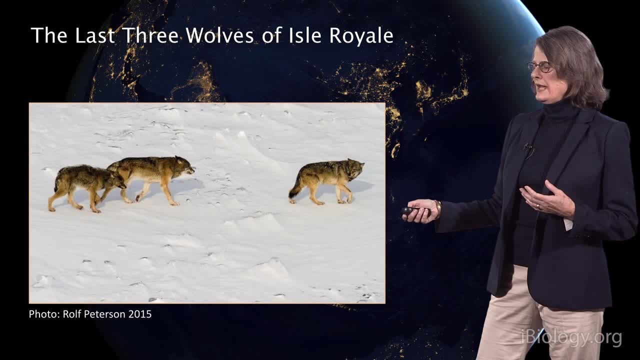 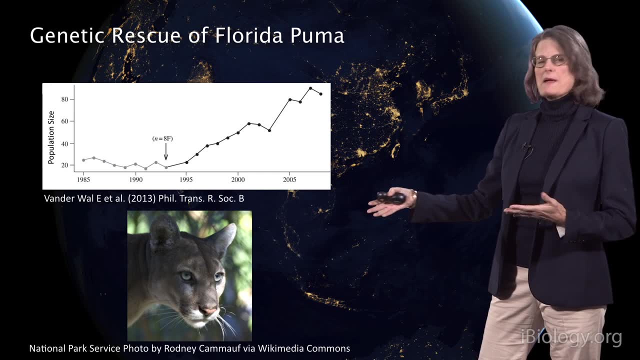 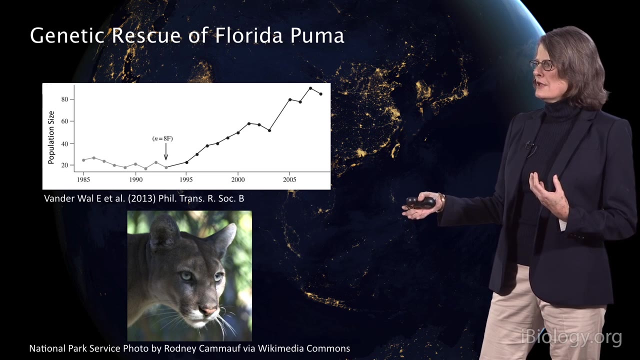 and clearly this, this wolf is, has been affected by inbreeding, So there is this possibility to rescue populations by bringing in some, some kind of new individuals to a population, and that, indeed, is what happened to the Florida puma. 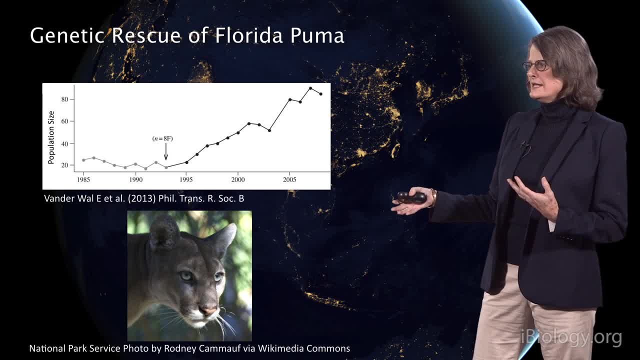 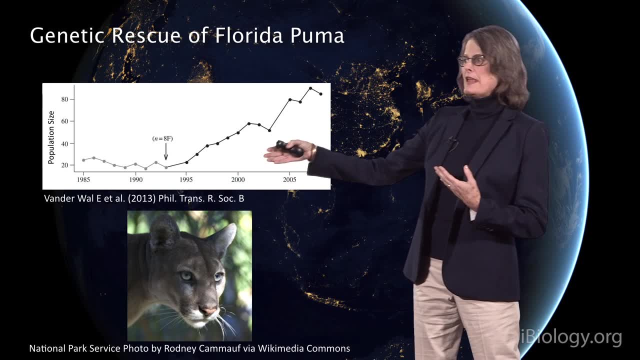 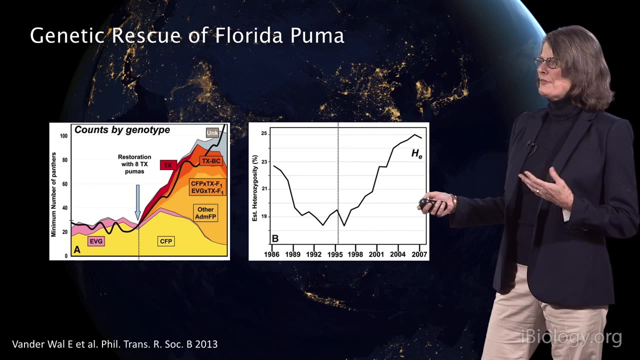 So in the mid-1990s, puma were brought in from Texas, and what you see in terms of the population size, which was on decline, is that they basically started breeding more frequently and so the population really bounced up in individuals. 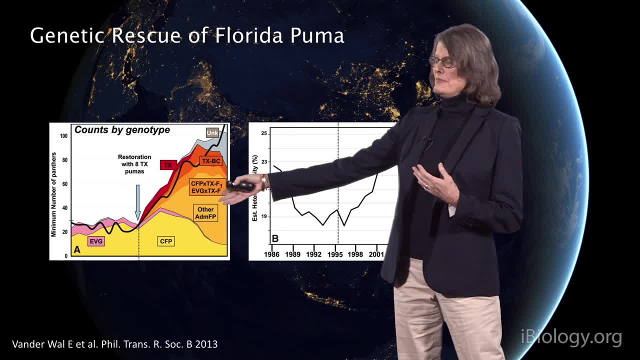 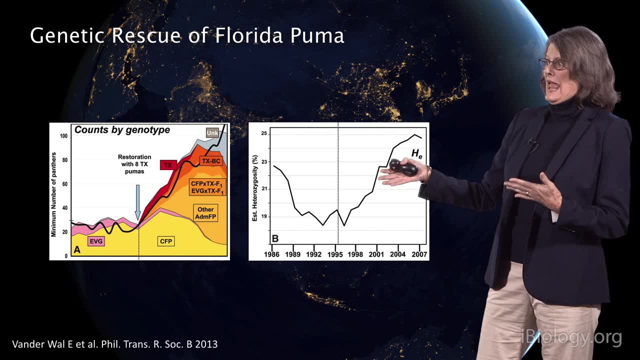 But there was also a rescue of genetic variation: These same, this eight, this puma. you see, before this time there's there's hardly any variation, and after that time there's an enormous increase in the amount of genetic variation in this population. 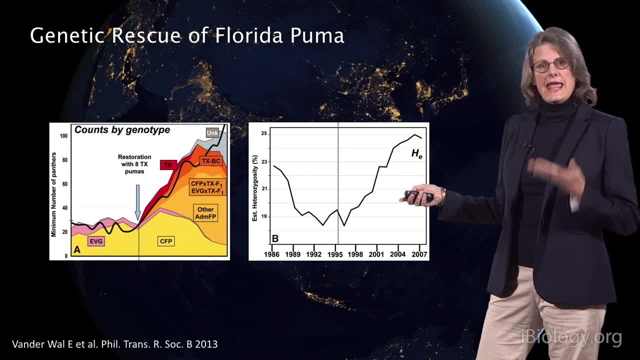 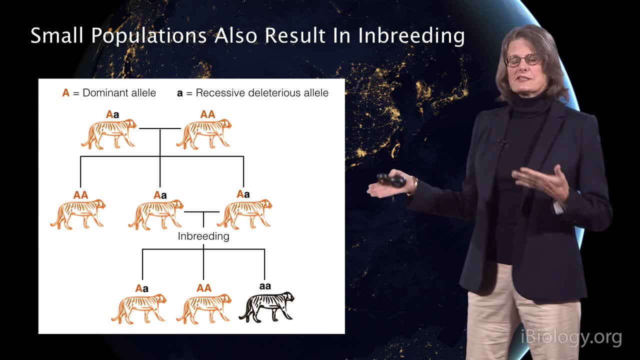 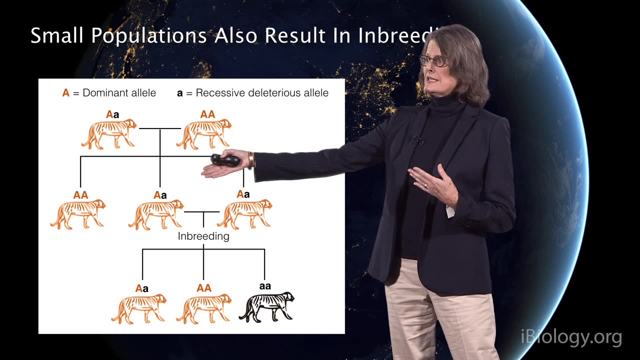 suggesting that there's been genetic rescue just by adding eight individuals from another healthier population. Small populations, then, to kind of summarize this part, small populations tend to result in inbreeding, And so- and this is because it brings out the recessive, deleterious genotypes- 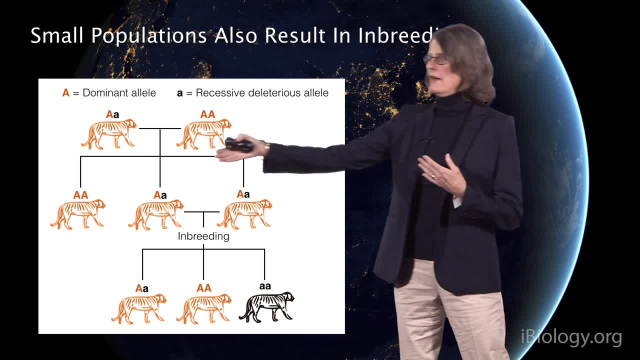 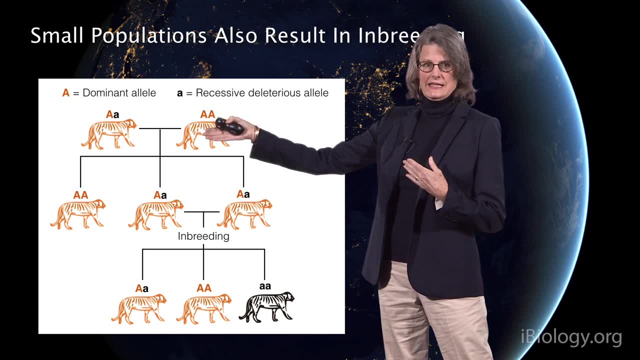 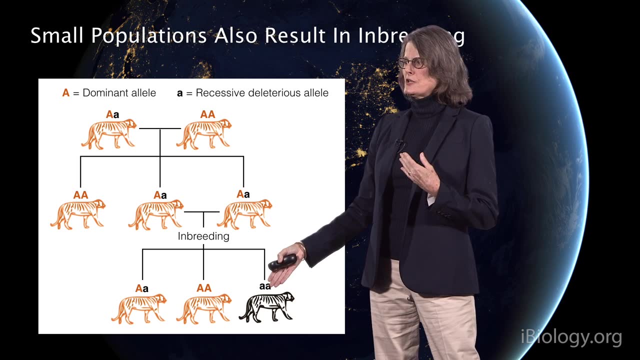 In this case you'll see this, this lineage showing this recessive allele that doesn't get expressed in the offspring, because there's always this dominant allele, this large A, that is overprinting it. When there's inbreeding, you have the opportunity to produce an individual that has both of 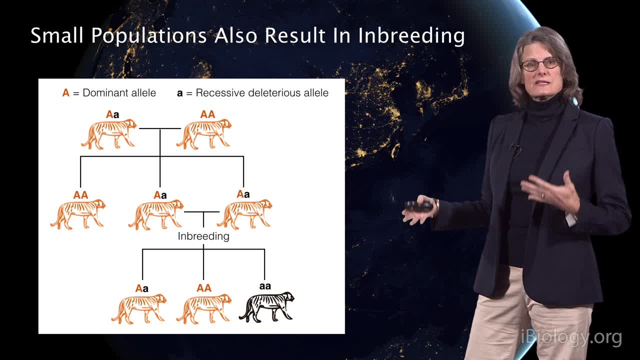 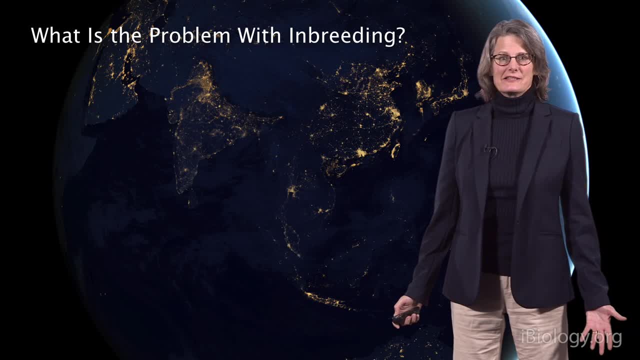 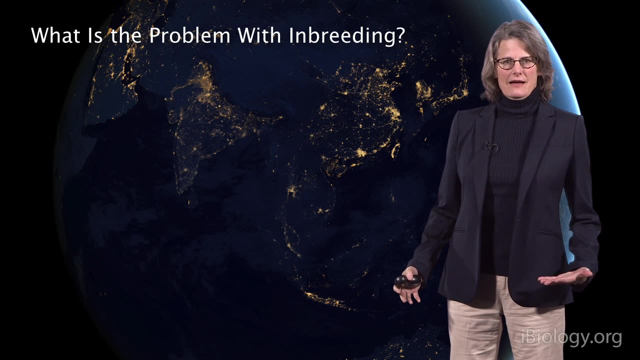 these recessive alleles, And what that means is that these deleterious phenotypes then become expressed. Okay, so what are these recessive, deleterious alleles? What do they result in? What's the problem with inbreeding? It turns out that the inbreeding creates a pretty typical list of problems with with. 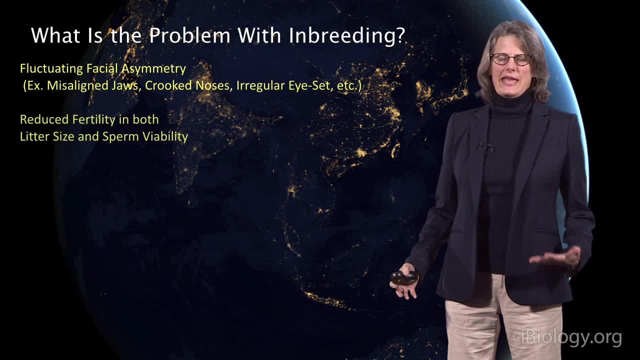 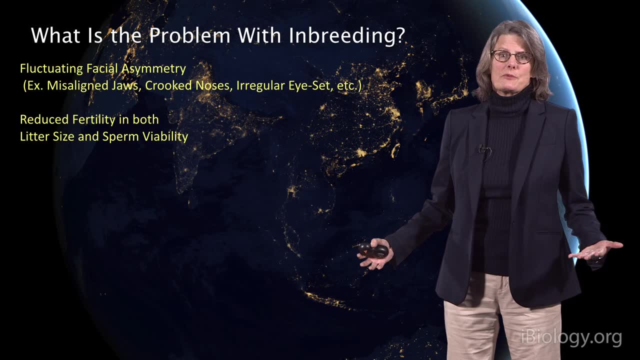 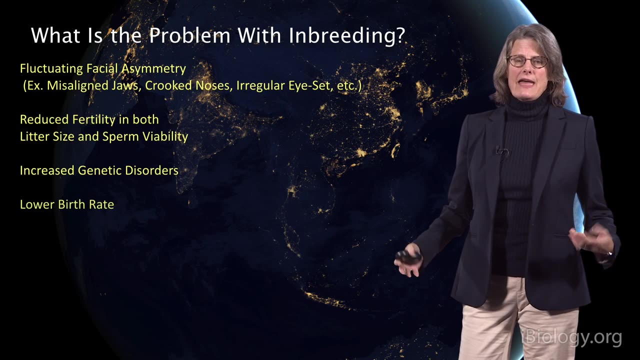 many animals. Their faces aren't symmetrical. they have reduced fertility, and this is true with both the number of offspring they produce and also whether or not their sperm are even viable. There are many genetic disorders, including Down syndrome, that show up in animals. 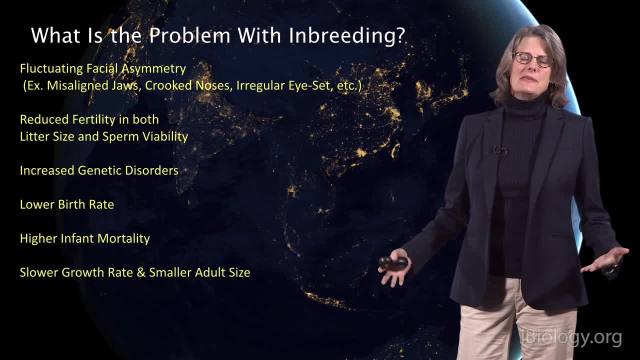 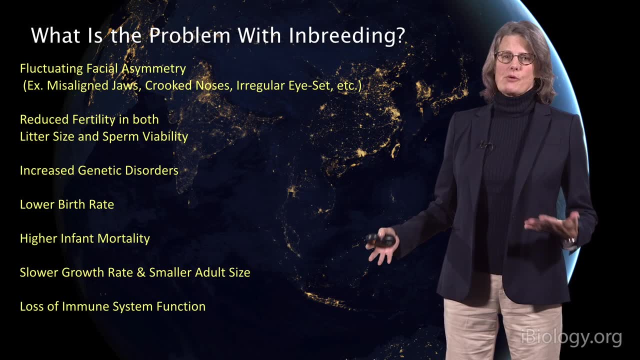 They have a much lower birth rate, higher infant mortality and because they have a slow growth rate, they also reach a much smaller adult size. And then, most importantly perhaps in this changing world is that they really lose a lot of their abilities to respond with their immune system. 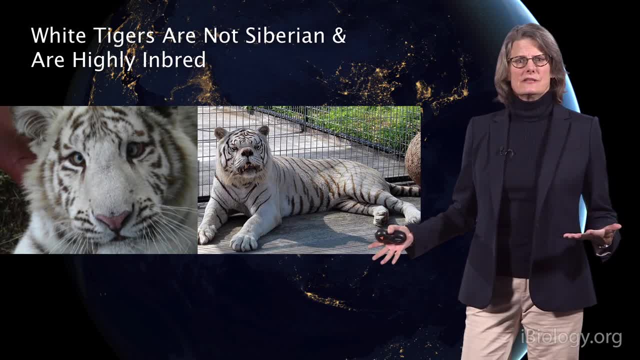 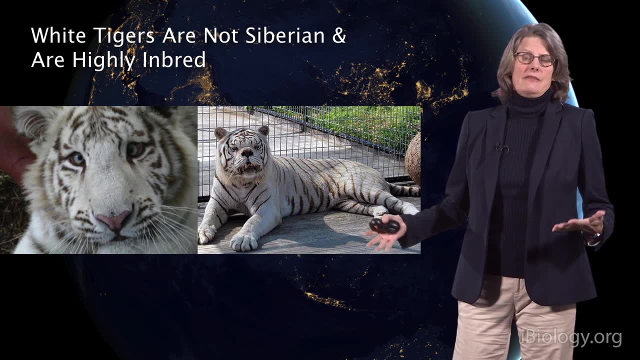 So I want to point out. here is an example in tigers. These are white tigers, White tigers. for those of you who don't know, white tigers are not Siberian. They look like they should be. They have this white coat. 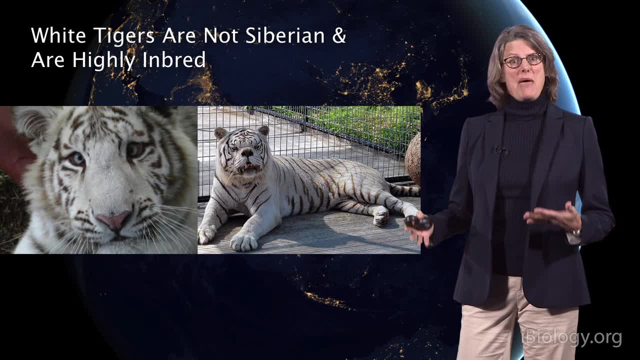 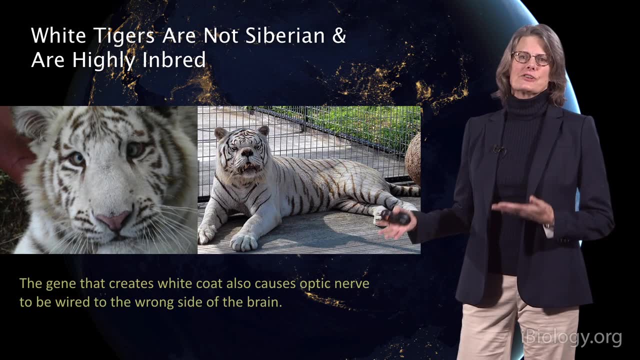 It turns out they're completely created in zoos. White tigers are actually Bengal tigers, they're from India and they've been highly inbred in zoos because people like white tigers. But it turns out the white coat is also associated with the same gene. 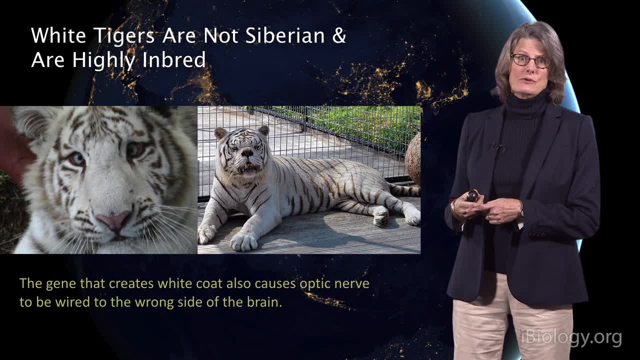 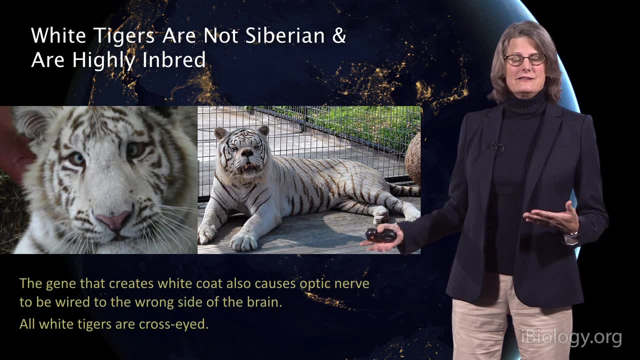 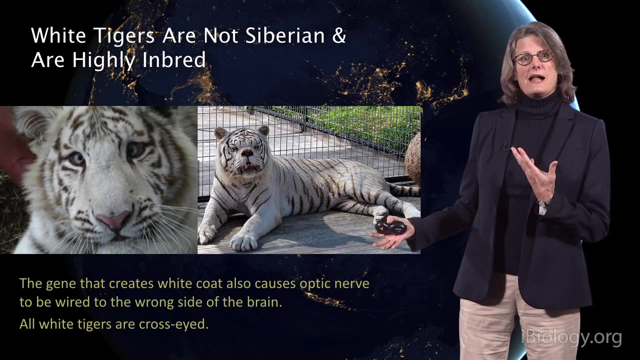 that creates cross-eyes in the individuals, So it crosses the optic nerve and so every white tiger that you see is cross-eyed. And you can see this other tiger here with a severely misformed face and a very asymmetrical face. He has a cleft palate.